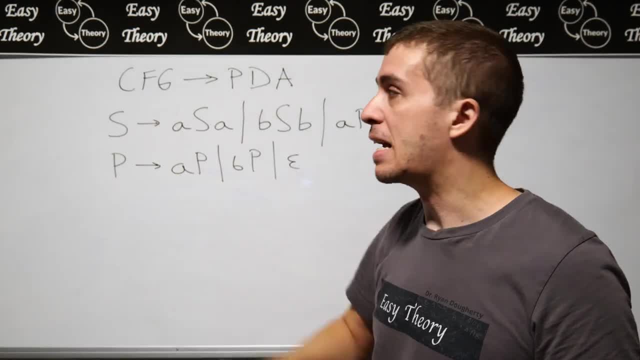 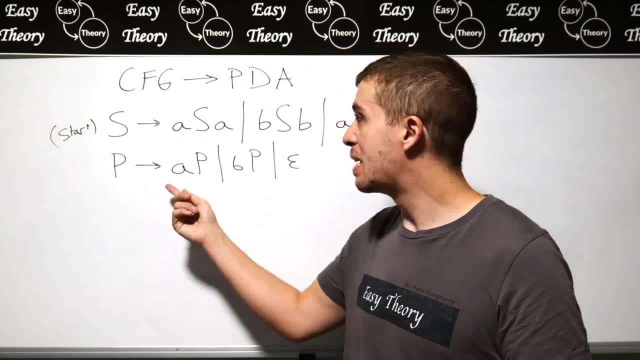 We have the start variable here, although I have not indicated that, which I should do, so I will indicate that this is the start variable. Of course, P could be the start variable, but it doesn't reach S, so it doesn't really make sense, but it's important to mark the start variable. 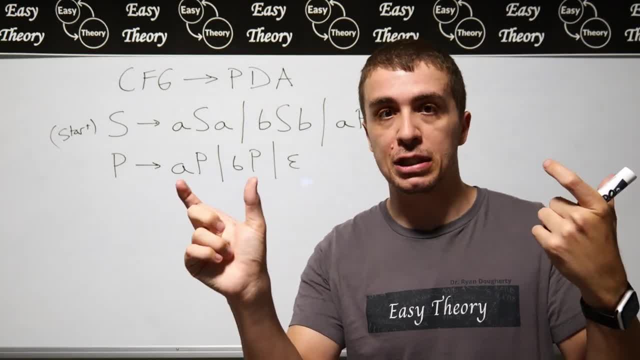 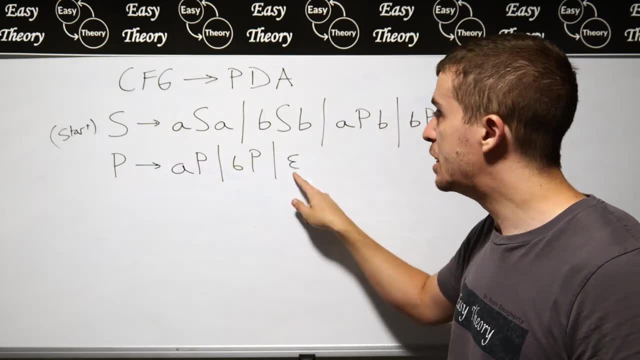 If we have a string that's not a palindrome, then the same distance from either end of the string must have different characters. In order for this grammar to make a string, we need to hit this particular empty string down here, because every other rule has some variable in it. We need 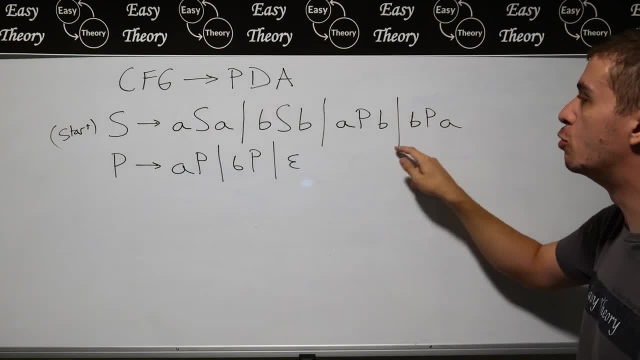 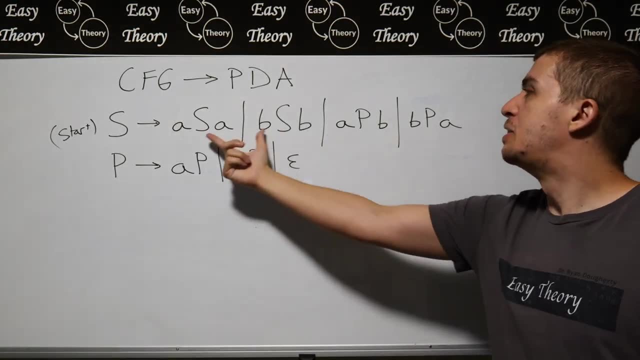 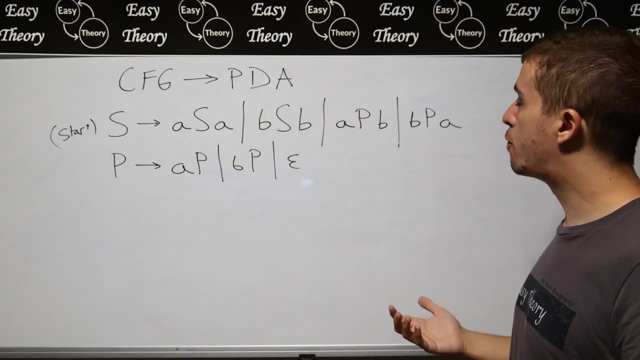 to get down here from S, which means we must hit one of these two rules, because these two involve S and that's not going to help us very much. But if we hit one of these two, since every single rule upstairs for S has exactly one character on either side. therefore, if we hit one of these two rules, 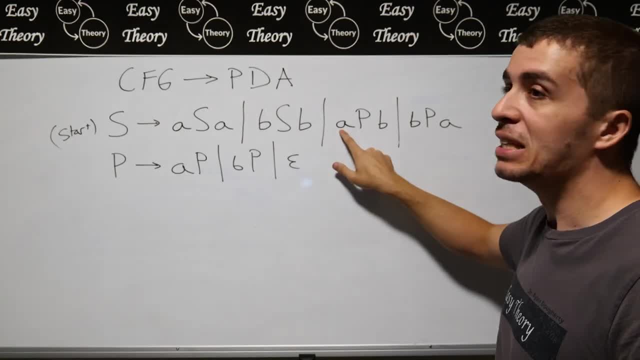 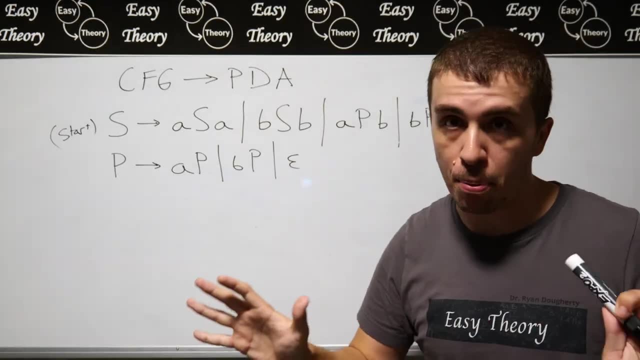 which we must do to make a string. that means that we have in the same position, on either end we have differing characters, and so therefore the string is not a palindrome, But it's not important that this grammar has that particular language. I 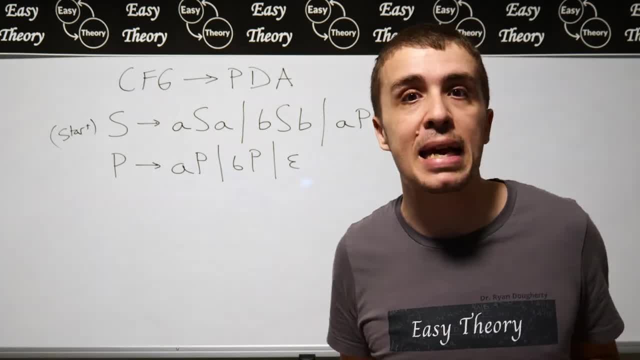 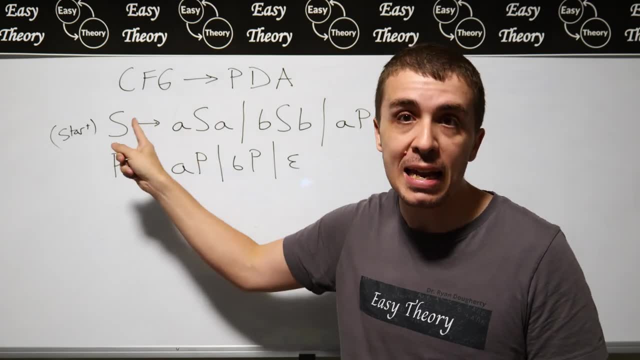 wanted something that is somewhat non-trivial. Obviously, there are many different PDAs that you can make, but it's important, when we talk about a conversion like this, to be able to apply it to any context-free grammar, not just this one. We could specially make a PDA for this grammar. 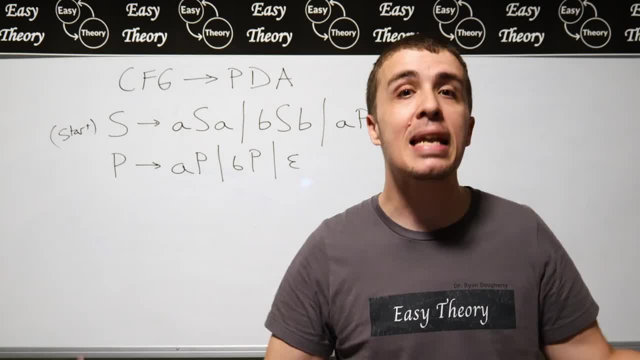 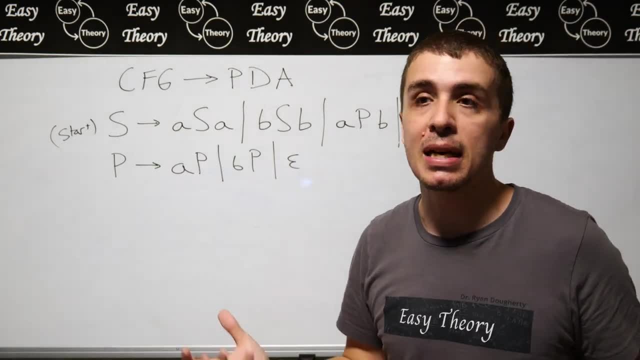 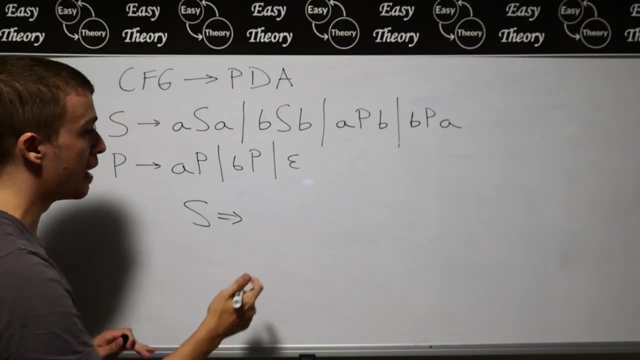 but I'm going to do a general conversion that works for any grammar, so you don't have to work with this specific one. If we think about what a general, context-free grammar does, what we do is we start with the start variable and then we apply a rule. So this double arrow means apply a rule. That means: 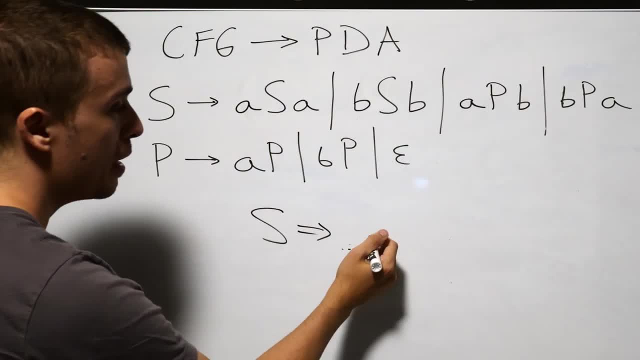 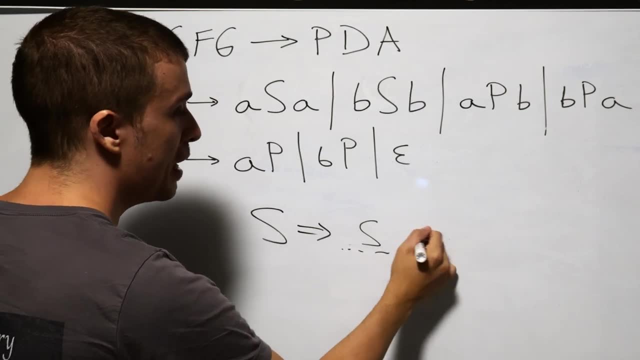 we're going to get something on the right-hand side from applying that rule, Then maybe there's an S in here, although it doesn't have to be. We could immediately jump to the P variable here. but let's just say there's an S, Then that means we're going to apply some rule. 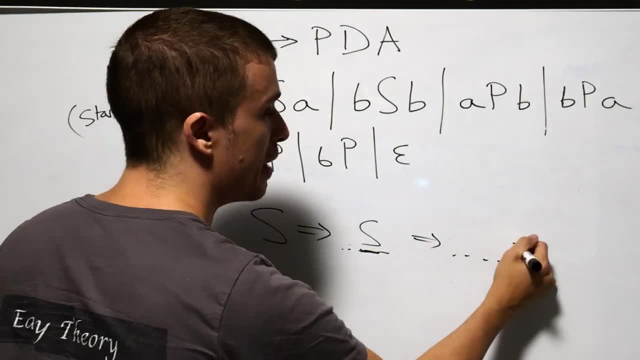 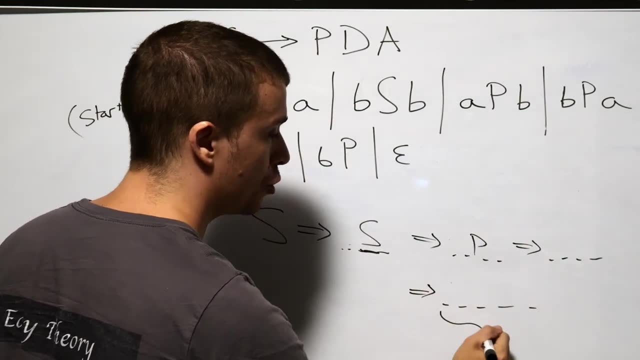 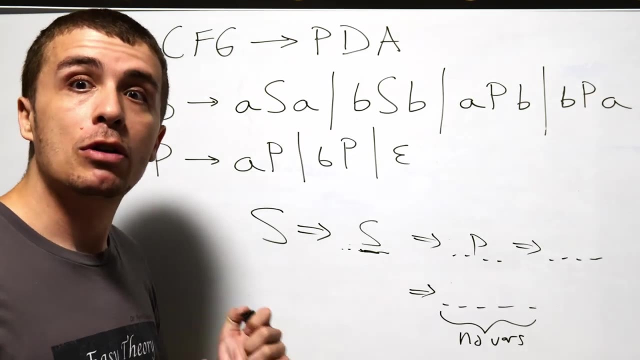 to this S, Then we're going to have something over here. Then we may have another variable- Maybe there's a P here. Then we just keep going until we arrive at some string which has no variables whatsoever in it. That's important, because the language of the grammar is the set of. 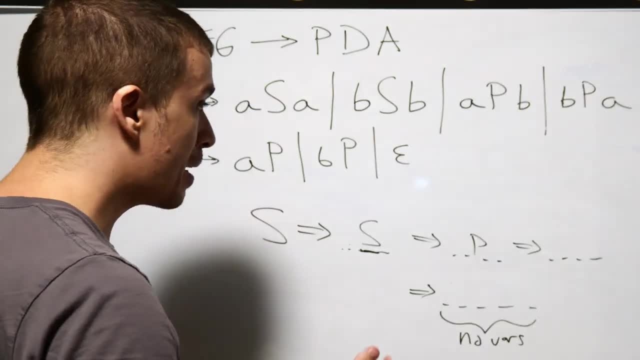 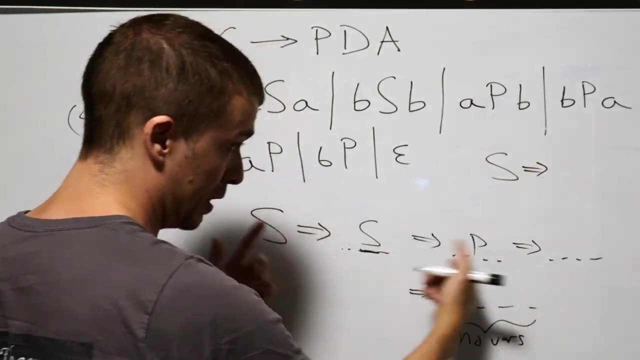 strings that you get that happen to have no variables in them. If we think about what a context-free grammar does, let's just imagine some particular derivation that we make. This is obviously called a derivation. If we have a derivation and let's say that we have an S variable right here, that's the. 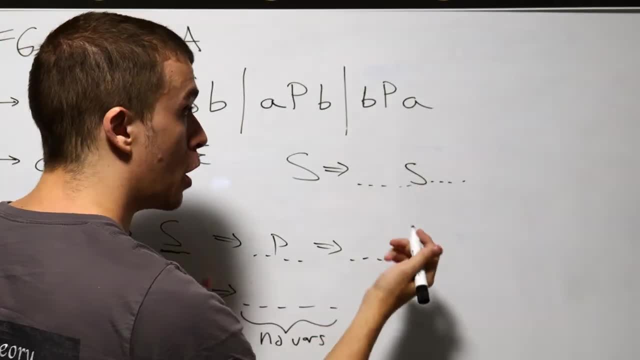 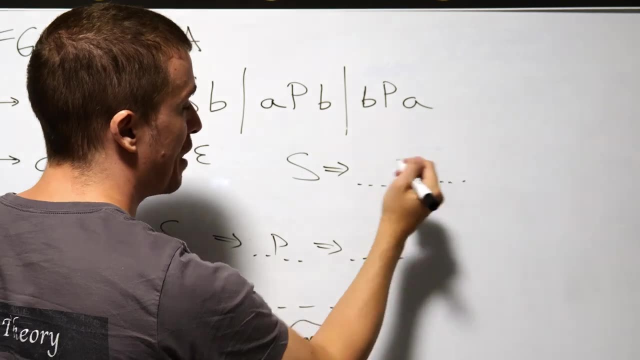 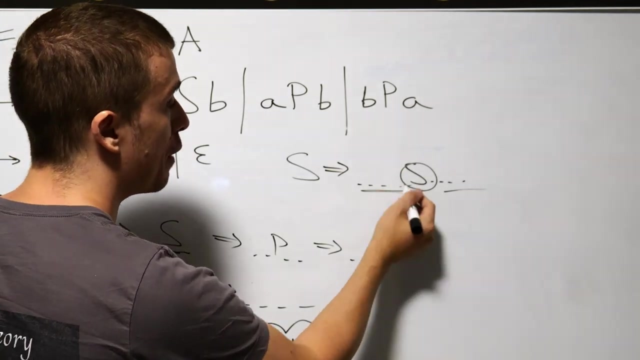 thing that we're going to replace. Well, if we have a context-free grammar, we're always replacing one variable with stuff. Therefore, we're going to replace that with stuff, But all of the other things on either side are not going to be replaced. Therefore, the stuff. 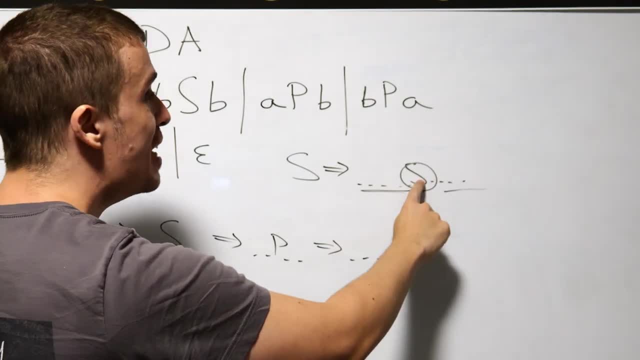 over here could be, in principle, anything. It doesn't depend where this particular S is in this right-hand side. So if we're going to have a context-free grammar, we're always replacing one variable with stuff, But all of the other things on either side are not going. 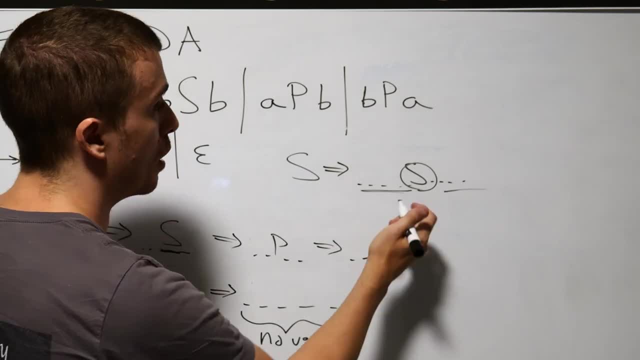 to be replaced. So if we have a context-free grammar, we're always replacing one variable with stuff. Therefore, this is the first variable that we're going to use. So what we can do to make this even simpler is to focus on when this variable S right. 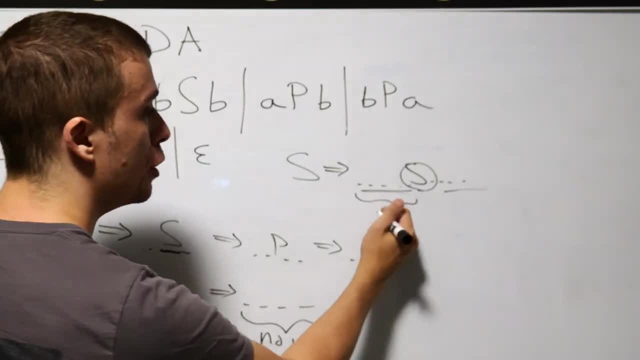 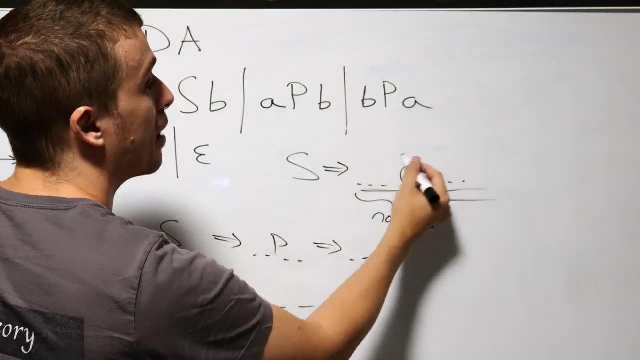 here- although it doesn't have to be- S is the first variable. So over here there are no variables whatsoever, And over here there could be, in principle, anything. But if we have the leftmost variable, therefore, we can always work with that without loss of generality. 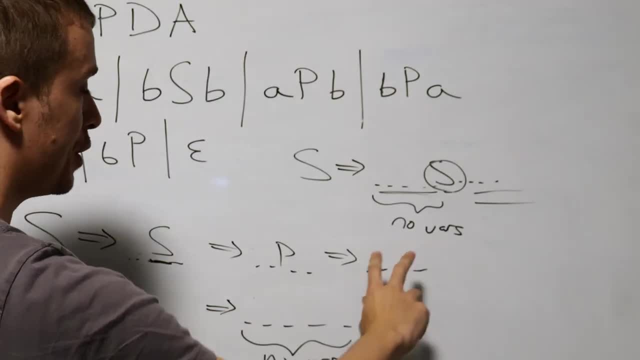 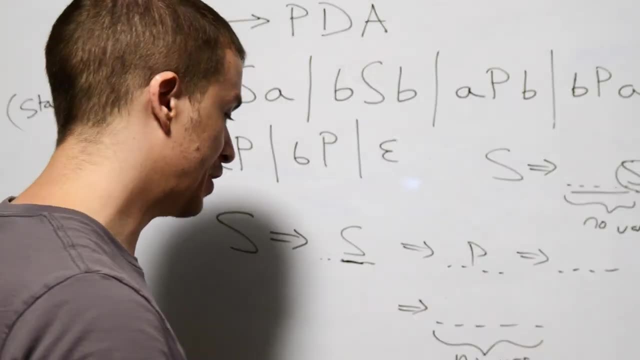 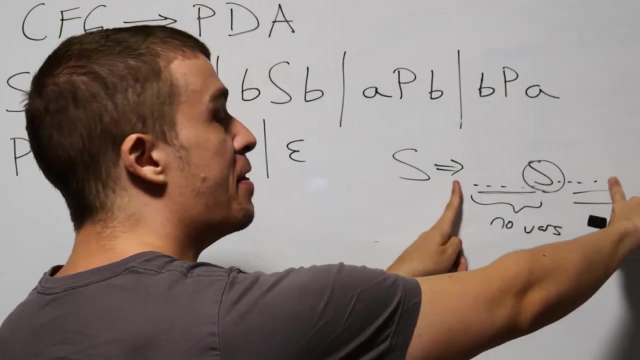 because we have a context-free grammar. If we focus on this, well, how do we get the to a PDA, which involves states and a stack and all of this kind of stuff? the idea is actually really, really simple, So all you have to do is to take this right. 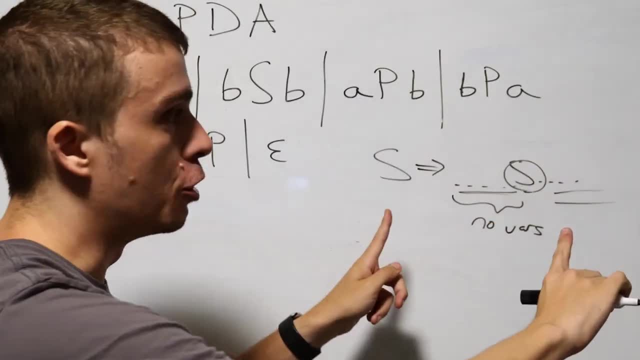 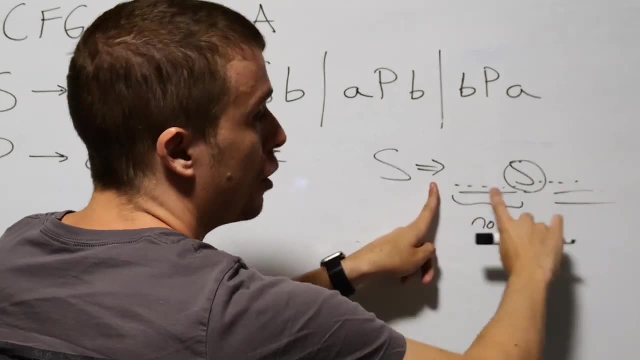 hand side and then just do a 90 degree change to it, And by 90 degree I mean literally 90 degrees, And what I'm gonna do is this right hand side. well, this is all the right hand side, but the right right end of this is gonna be coming. 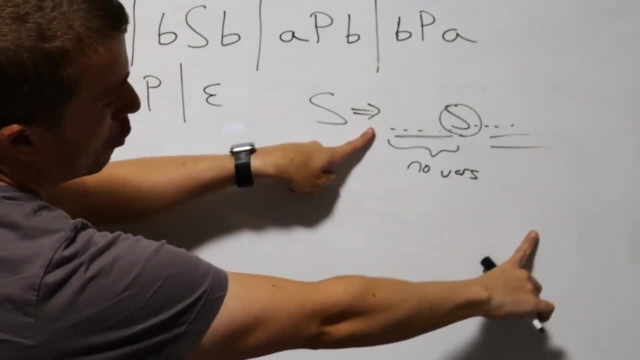 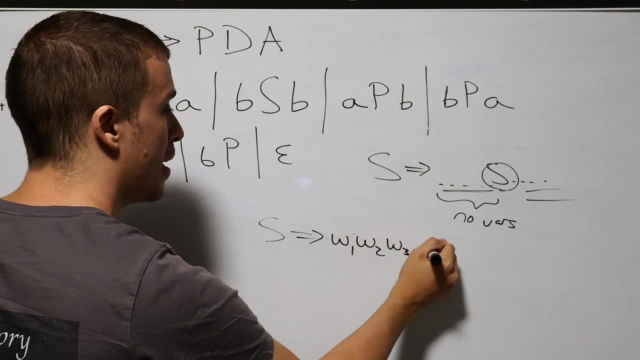 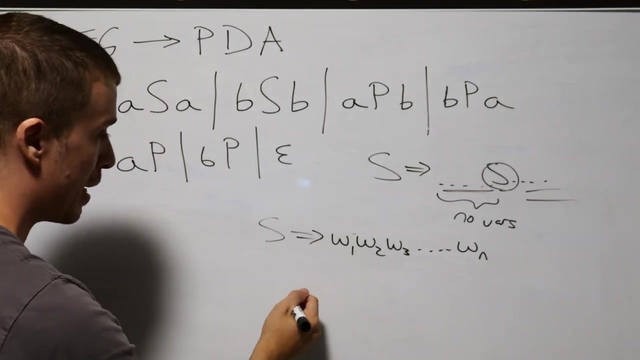 down to the bottom here. So notice, I do this 90 degree transformation. Let's say that this right hand side was W1, W2, W3, up to Wn, where these could be variables or terminals, it doesn't really matter. Then what we're going to do is the goal. 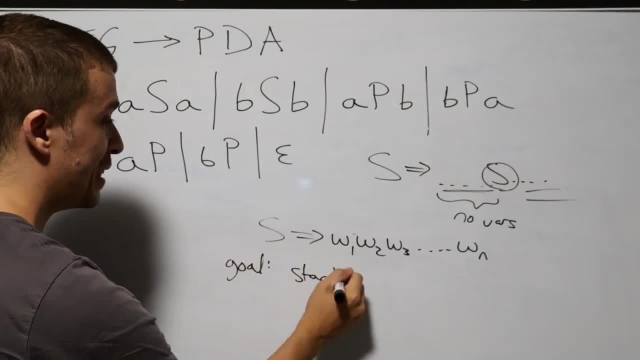 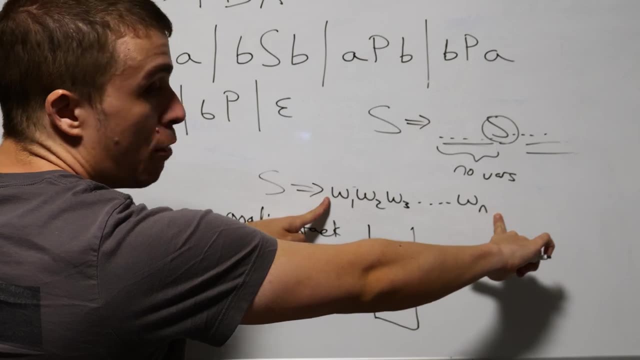 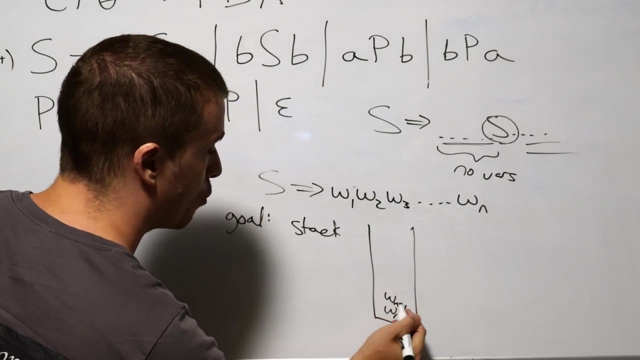 being to have a stack, because that's what the PDA needs with this particular configuration. Take this right-hand side right here and I'm gonna move my right hand side finger down 90 degrees, so now it's at the bottom. The wn is going to be at the bottom, then n minus. 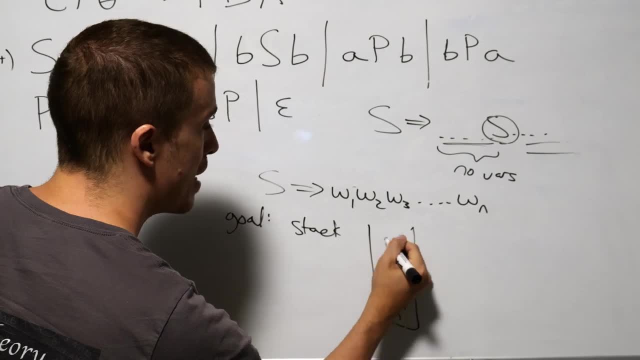 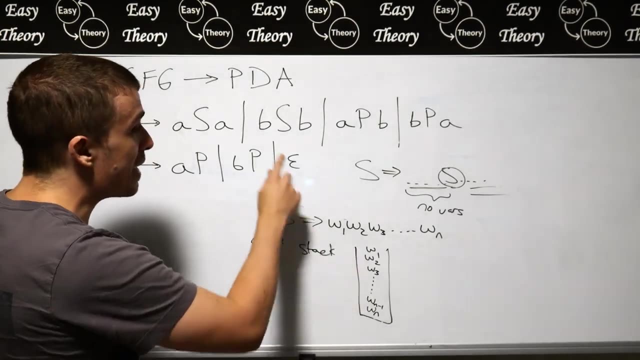 1 above that and then etc, up to w3, w2, w1.. So w1 is up top here. And why is this important? Because the PDA is going to be reading characters left to right. So if this is the string we eventually make, 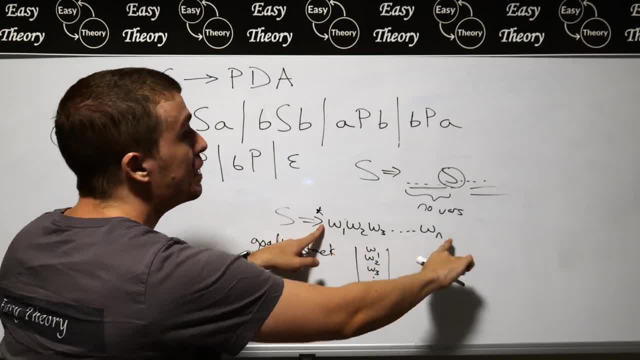 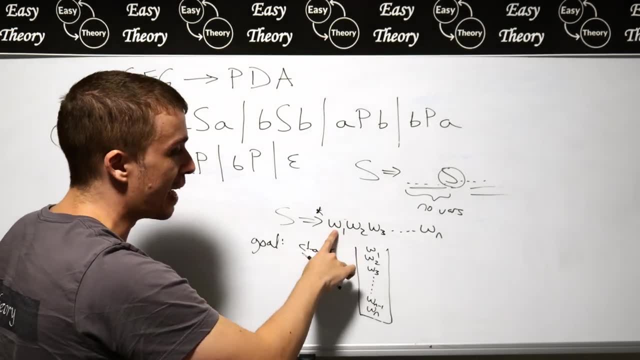 so this is not just one rule application, but many. If this is the eventual string that we make, then that means that this thing is the first character that's going to be read in the PDA, which means that if we're going to be storing this on the stack and then working with the stack as we 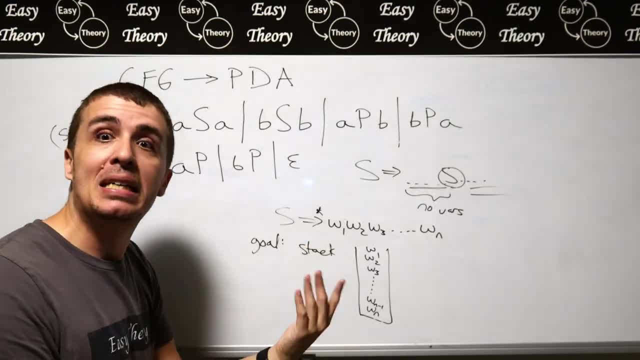 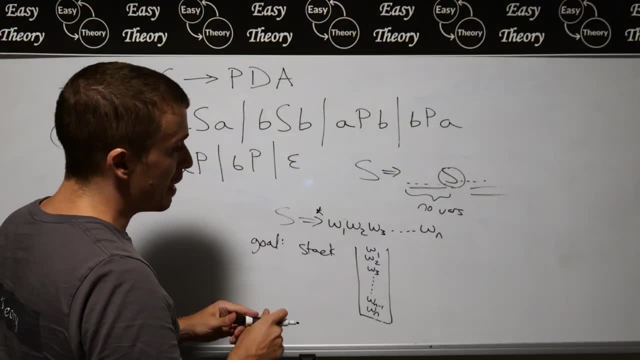 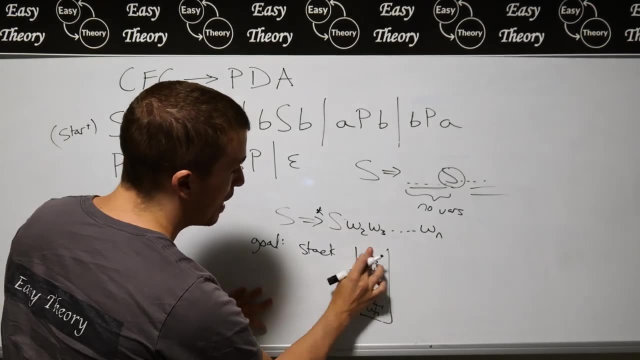 go, then this thing must be at the top of the stack, because that's how stacks work. You can only pop off the very top of it. That's how the general procedure is going to go. Well, the problem is well, what if this very first thing is a variable like s or something? Well then, obviously up here this. 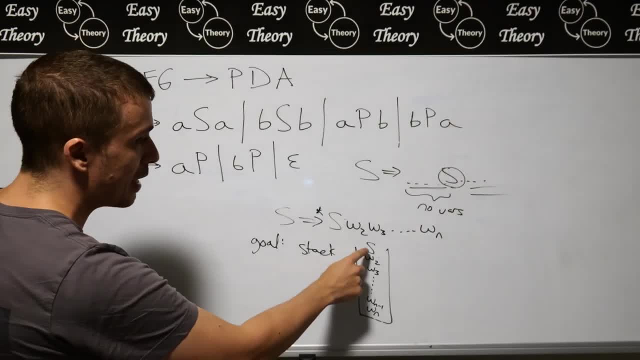 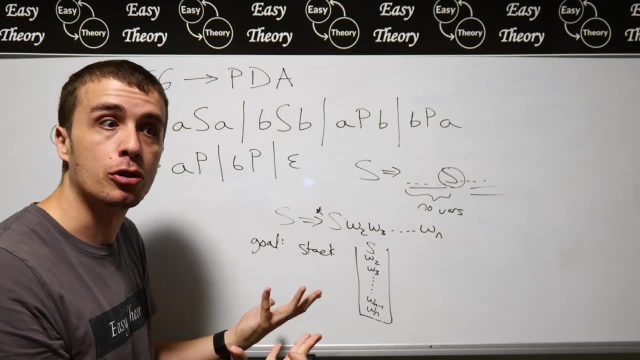 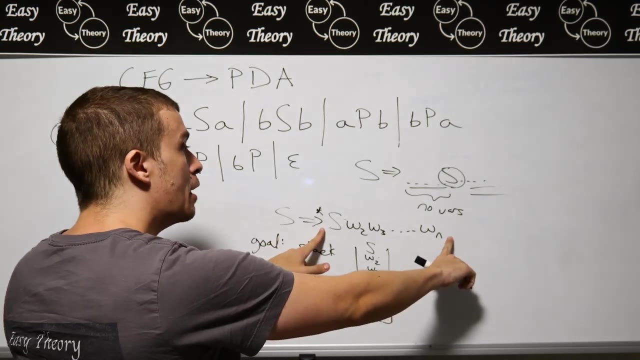 is going to be an s. Well then, what are we going to do? Well, we can't just read off of the input, because the input string has, in this particular case, a's and b's, but in general terminal, whereas here we have a variable. So, if we have a variable, whenever we have some a variable in the derivation, if it's. 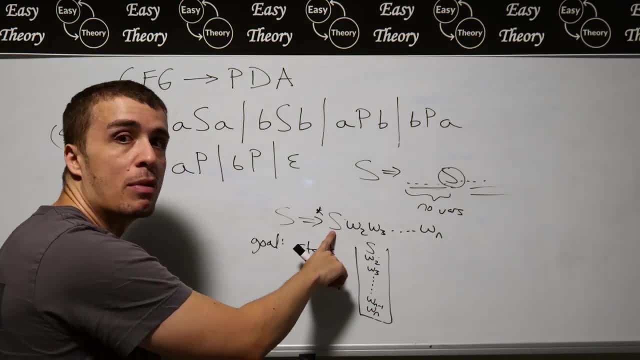 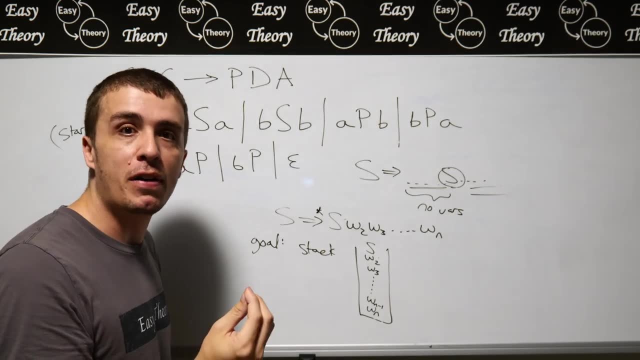 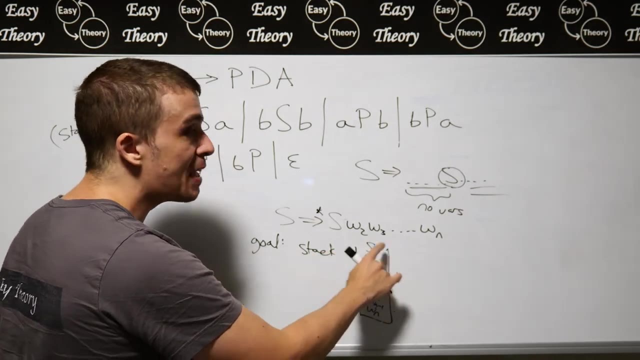 up at the top in the stack and that's coinciding with this. that means that there's nothing to the left of this s right here, which means that it's the left most variable and therefore we can apply some rule to it. So, the goal being in the PDA part, if we see a variable upstairs, let's 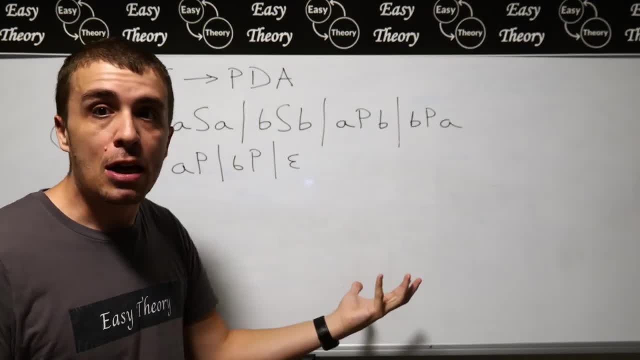 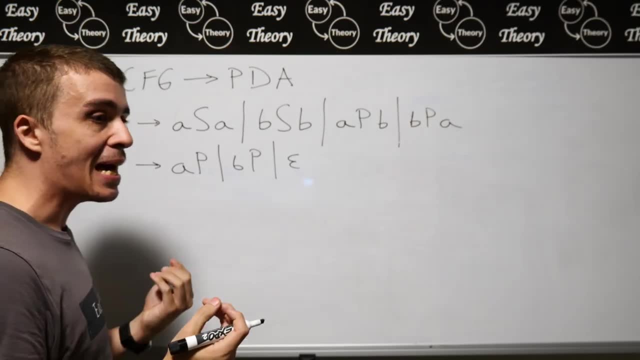 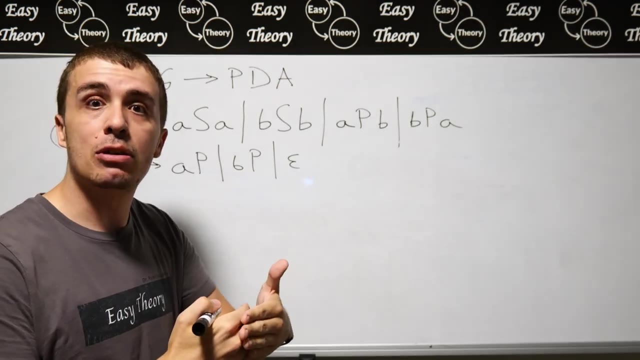 apply a rule to it: Every single derivation in any context-free grammar whatsoever always starts with the start variable, obviously, But the PDA stack doesn't have anything on it whatsoever to start with. There are some textbooks that have some kind of preliminary character at the top. 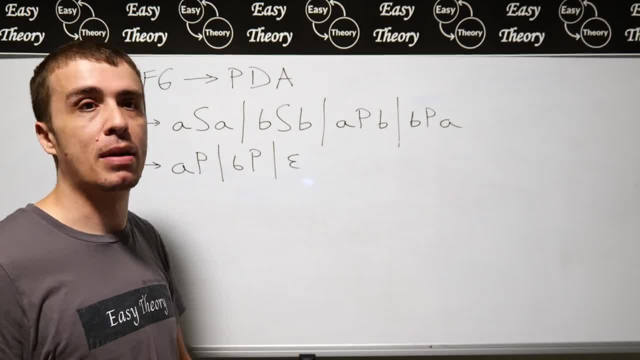 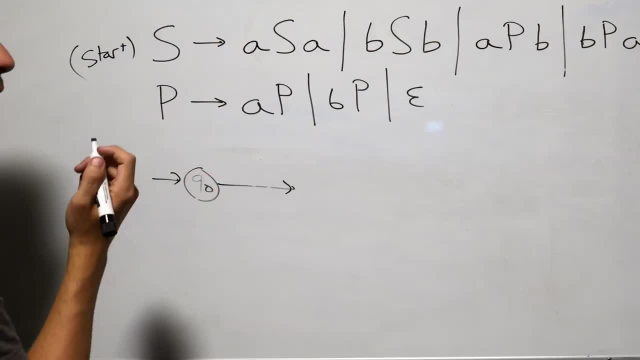 of the stack. but let's assume that there are no characters at the top of the stack, but then we need to put something on. So what I'm going to do is I'm going to have a state q0 right here. so, on this first transition, what I'm going to do is I'm going to read nothing. The way I'm going to format. 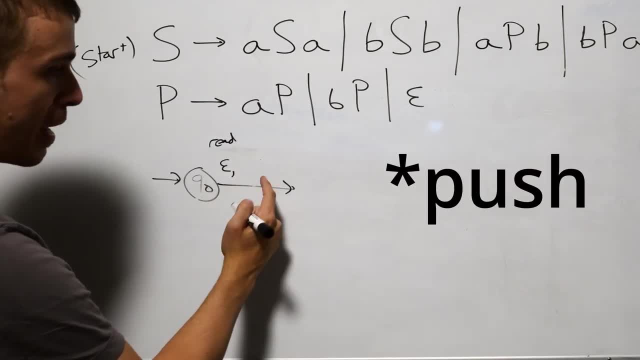 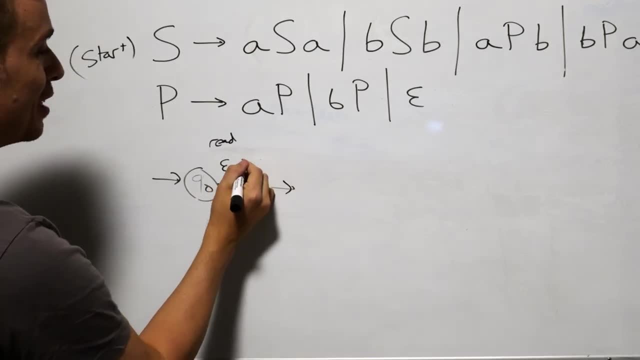 my transitions is: read first, then pop and then write. I'm going to read nothing here. Well, I can't pop anything here because the stack's empty and then that would be kind of pointless, So I'm going to pop nothing. so this is the pop one. so pops here, reads here, and then what I'm going to. 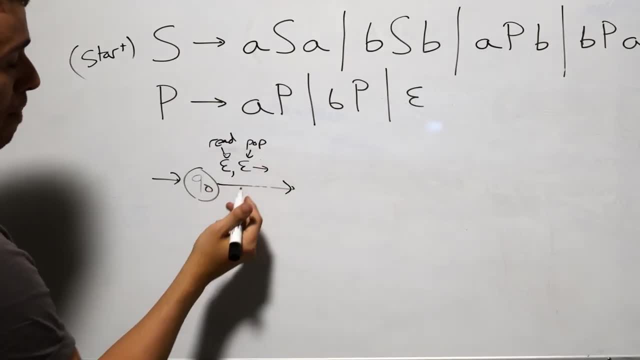 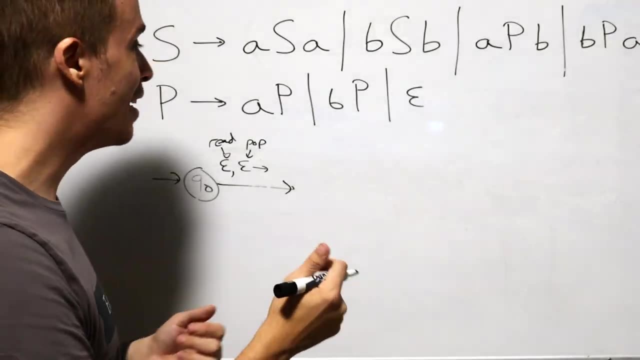 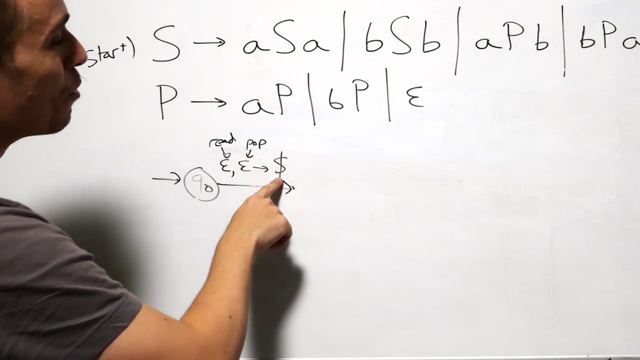 push This arrow means after the read and pop happened, which happened to be doing nothing here. then I'm going to be pushing something. I'm going to be pulling something out of a little hat right here and I'm going to be pushing on a dollar sign because I want to get rich, obviously, But the 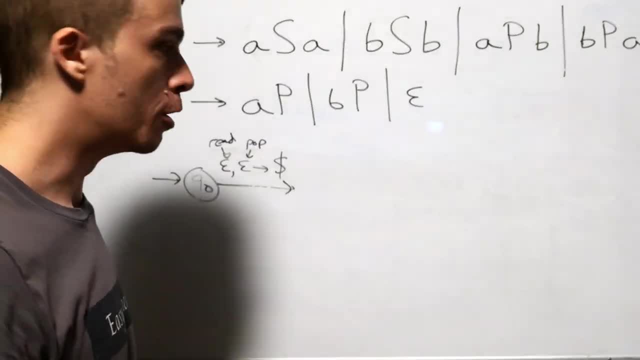 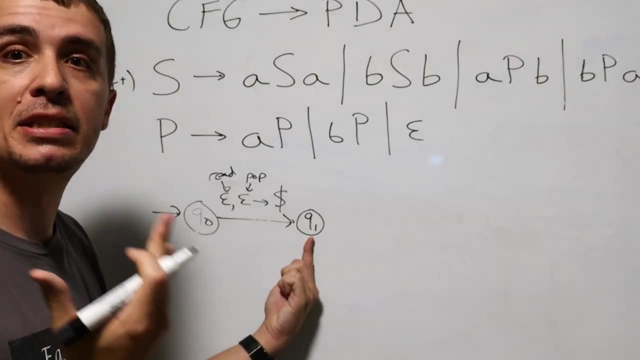 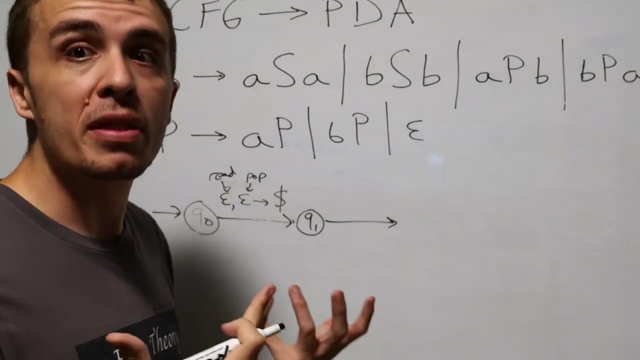 real reason is that this is going to come in handy. later. I'm going to go to a state right here, q1. so at this point right here, the only thing on the stack is the dollar sign, obviously. But then let's get into the meat of the business, and here we're going to start the derivation and every. 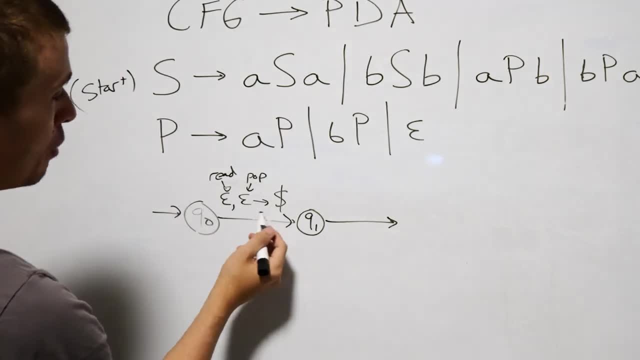 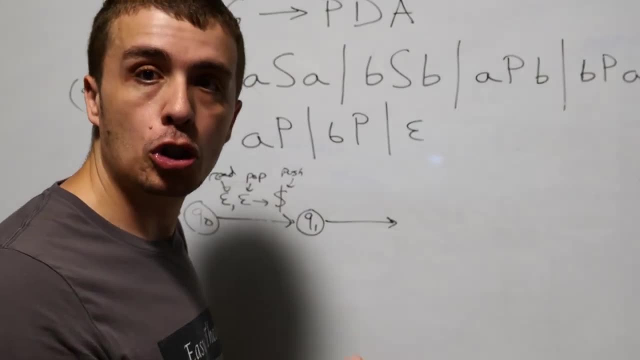 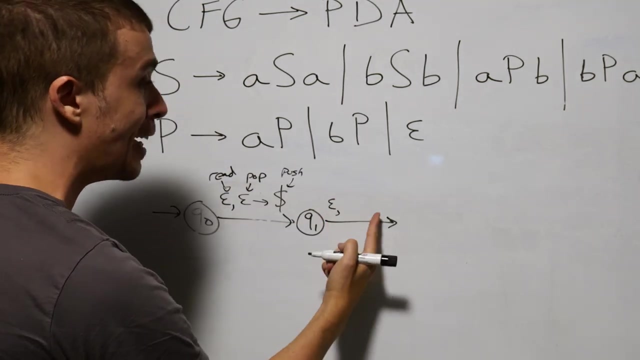 derivation starts with the start variable, obviously, so I'm going to do exactly the same thing. I forgot to say this is push. I'm gonna do exactly the same thing, except I'm gonna push the start variable of the grammar, which happens to be s in this case. But whatever the start variable's name is, that's. 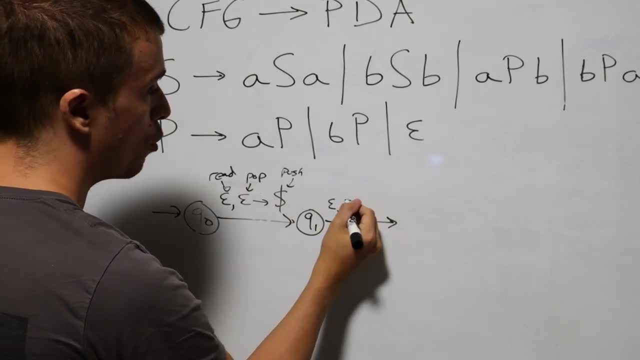 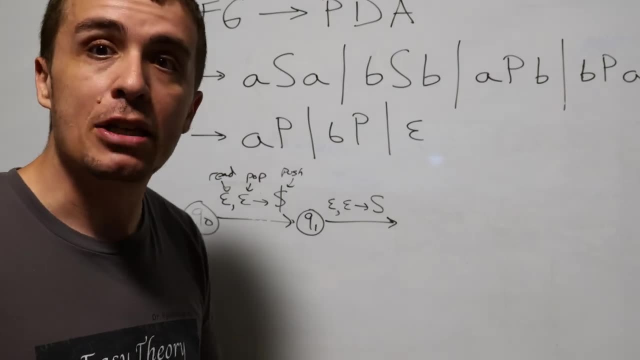 what's going to be coming here. So I'm going to be reading nothing, I'm going to be popping nothing and the start variable, which happens to be S here, If it was called X in your grammar, it would be X here. And then now I'm going to go to a state, I'm going to call 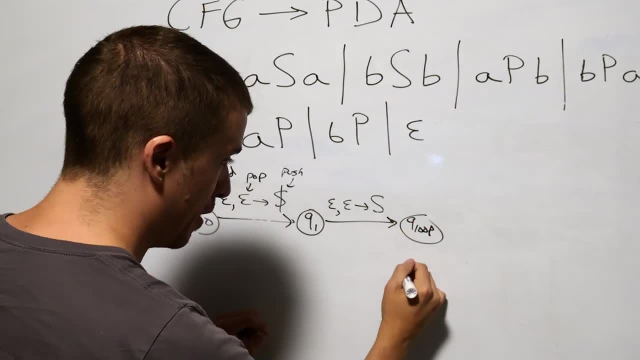 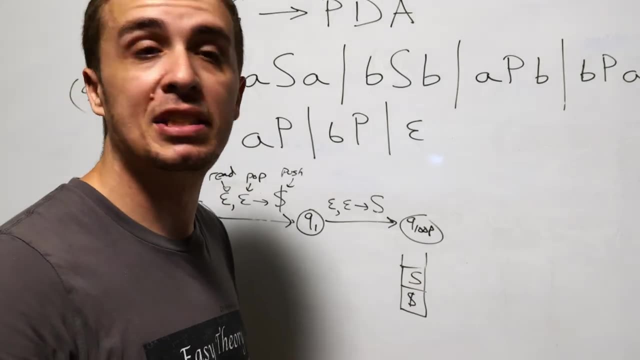 Q loop. At this point, right here, at this particular moment, we have this dollar sign at the bottom and S at the top, And that's all that's in the stack so far. Well, what are we going to do here? We're going to have this state be representing. 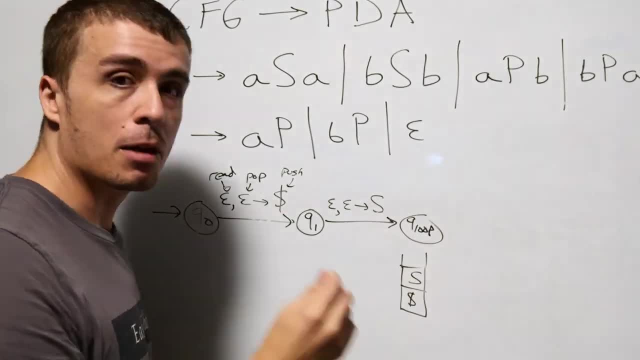 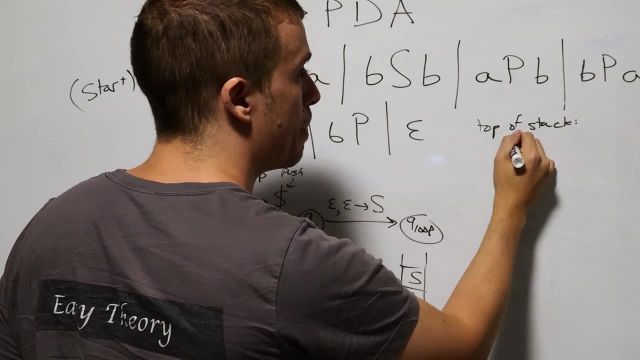 look at the top of the stack and then do something. The top of the stack can be one of three things, So the top of the stack can be one of three things. I'm going to write some notes right here, So it can be either a terminal, obviously. 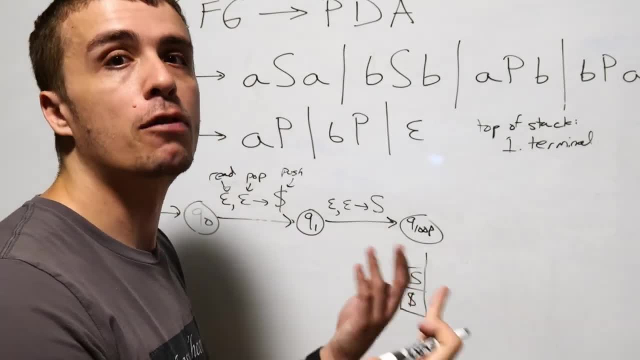 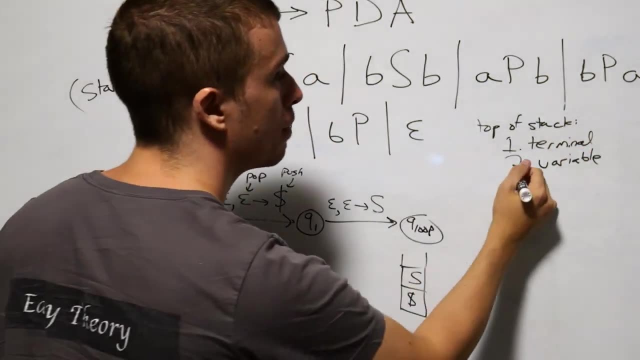 because we're going to be simulating a derivation and derivations involve terminals and variables. So there can be a variable at the top of the stack, in which case there is right here. Or three, we can have the dollar sign at the top of the. 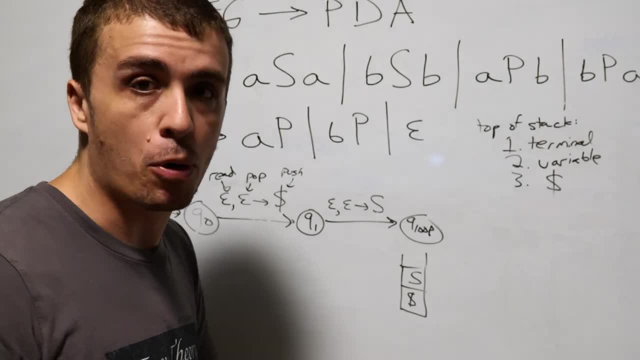 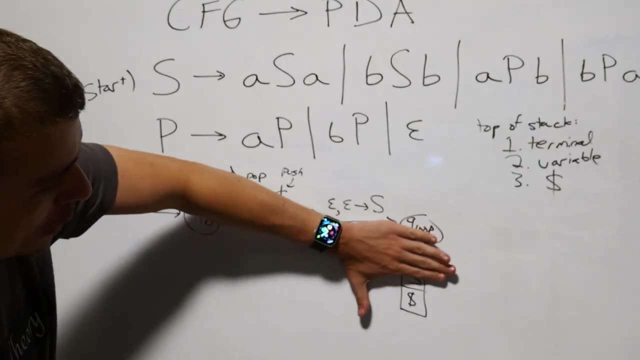 stack. Well, if the dollar sign is at the top of the stack, we're never going to be putting on another dollar sign. This is the only one. Apparently, I don't want to get that right, But if the dollar sign is at the top, that means that there's nothing above the 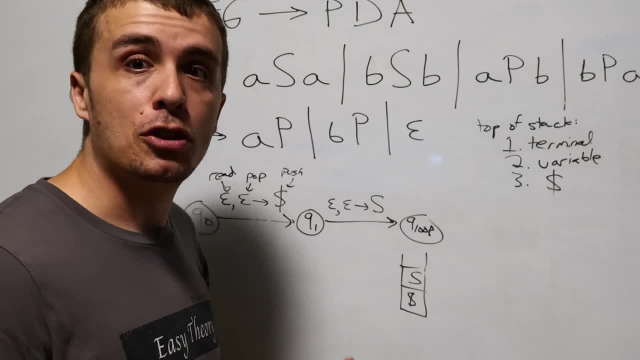 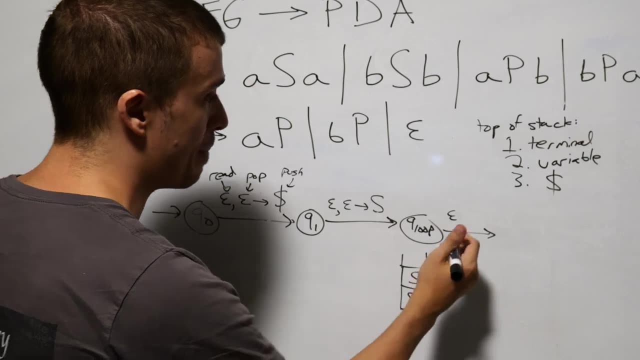 dollar sign right now, which means that there's nothing left to look at anymore, And so, therefore, we're effectively done with the computation. I'm going to do a similar type thing, but I'm going to pop off the dollar sign, which means that I'm 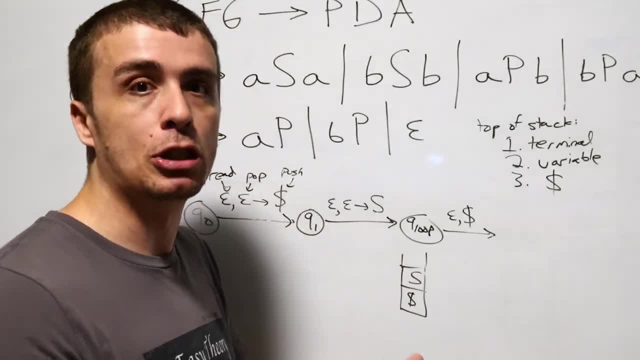 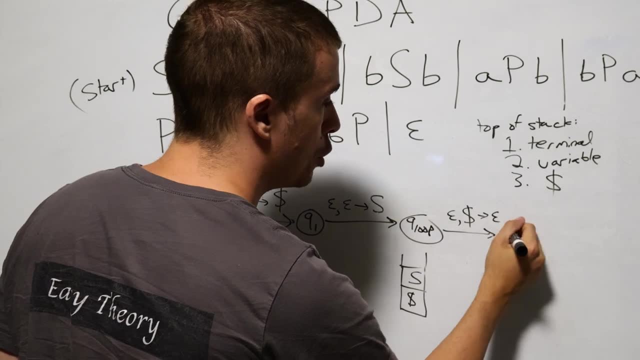 observing that there's a dollar sign. I need to do this transition only when there's a dollar sign on top And I could push something. but there's no point I'm going to do a final state here. So the final state is saying we're done at. 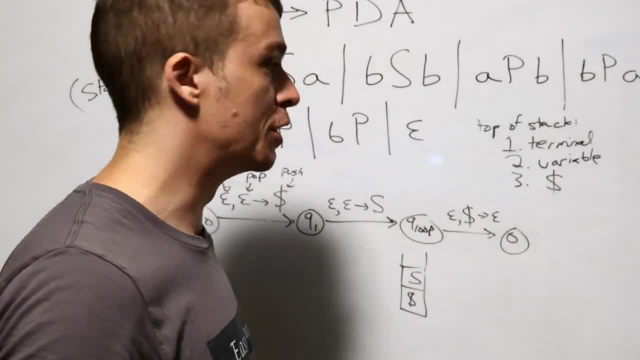 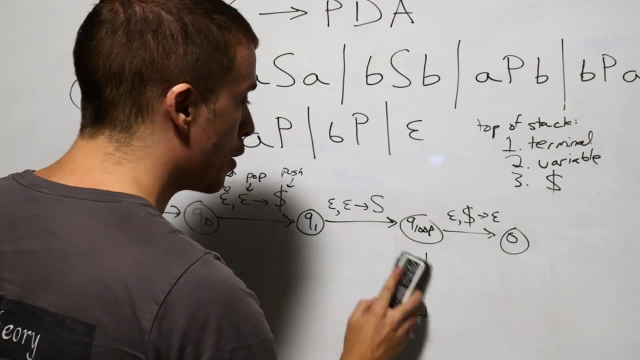 this particular moment, and this will be the only final state of this machine- We need to actually verify that this actually does the right thing. but that involves fixing the rest of the machine. What do we do in the other cases? Well, if there's a variable at the top of the stack, that's because we're trying to 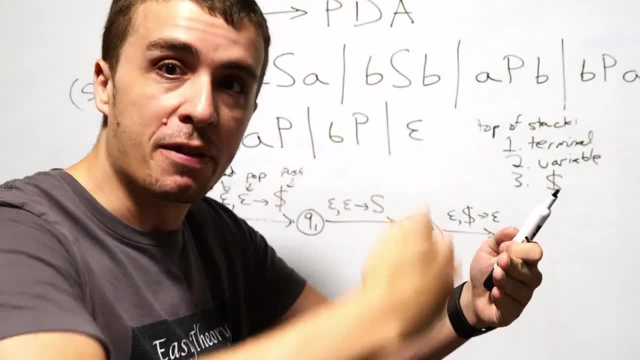 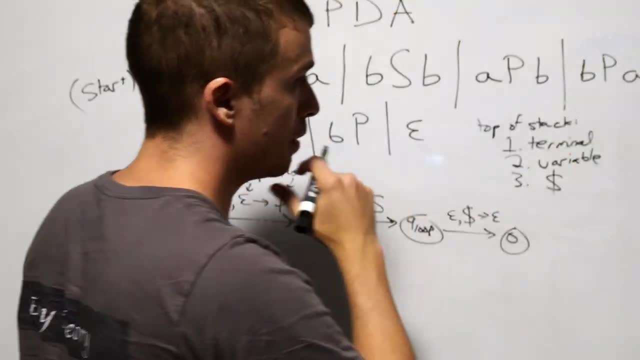 simulate a derivation and then, therefore, if we have a variable at the very beginning, that means that we need to apply a rule to it it. But I'm going to skip that for now. I'm going to talk about the terminals first. So if there's 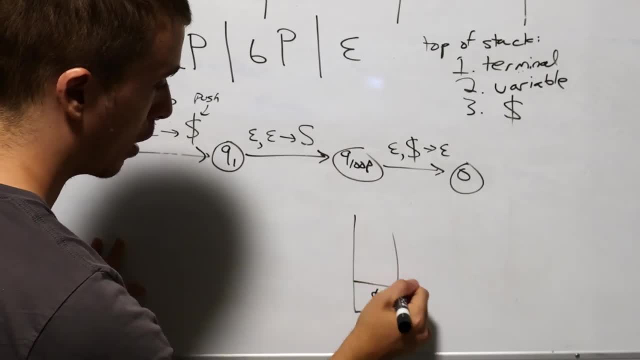 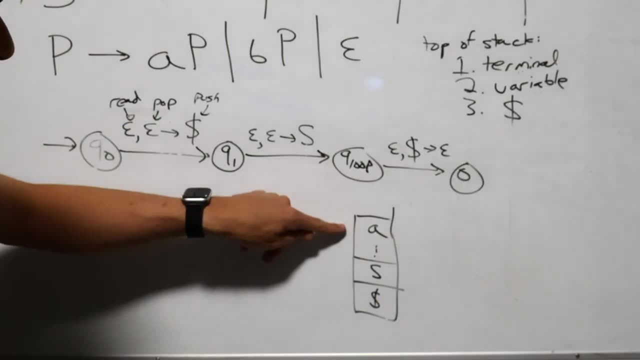 a terminal at the top of the stack. let's try to just see what that would look like. So let's say that there's S here and then maybe some other stuff, And then let's say that there's an A up top. Well, since it's a context-free grammar, I can't actually apply a rule to a terminal, because I can. 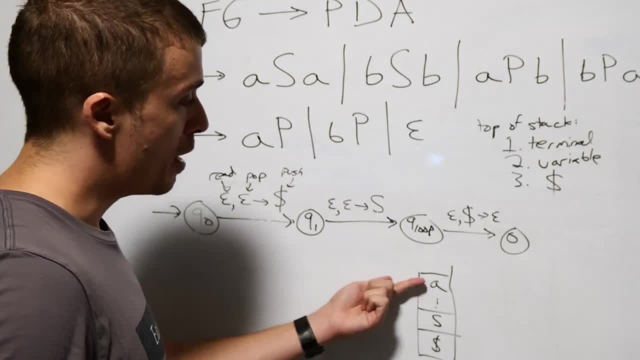 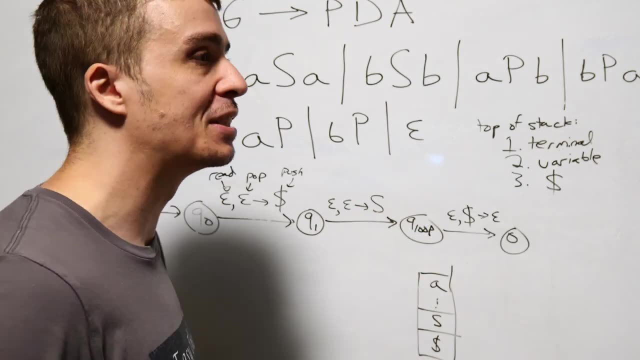 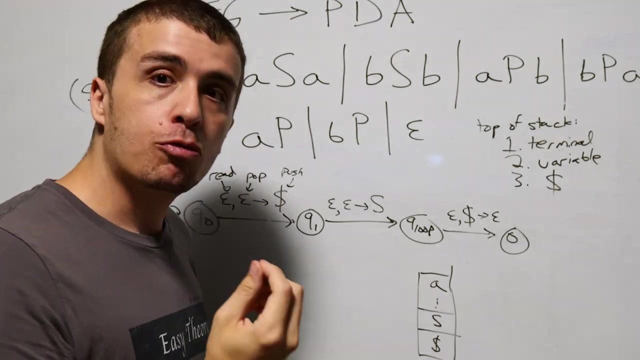 only apply rules to variables, And so therefore, this A is going to be permanently fixed in the grammar's derivation, because it can never be replaced. In other types of grammars it could be, But in a context-free grammar it can't. What can we do here? Well, since we're reading off of 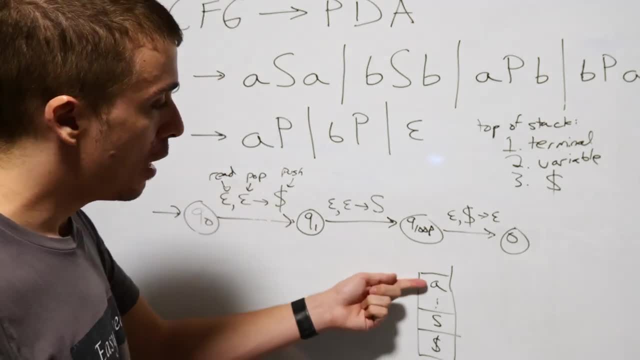 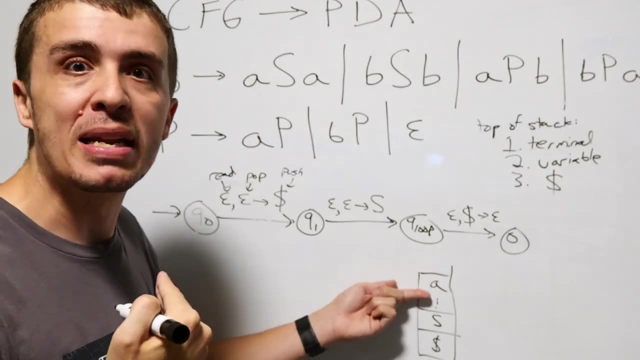 the input in the PDA. we can just say, well, if there's an A at the top of the stack and we are reading an A off of the input or we desire to read an A off the input, we can just say: 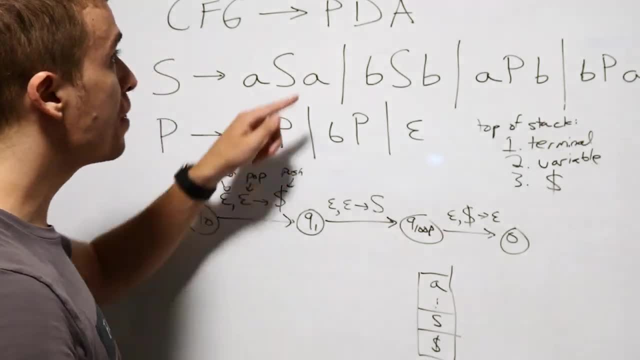 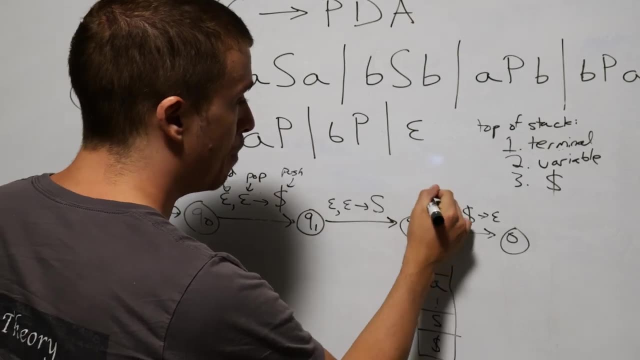 let's do both of them at the same time, Because we want the PDA's language to be identical to the context-free grammar's language, And so what we're going to do is a bunch of self-loops right here- although they don't have to be self-loops, but it's a lot easier. I'm going to do a read and a. 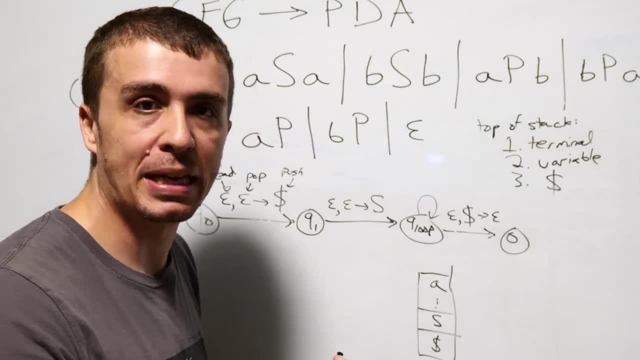 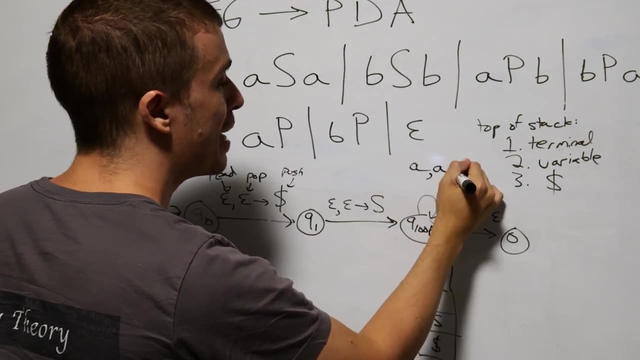 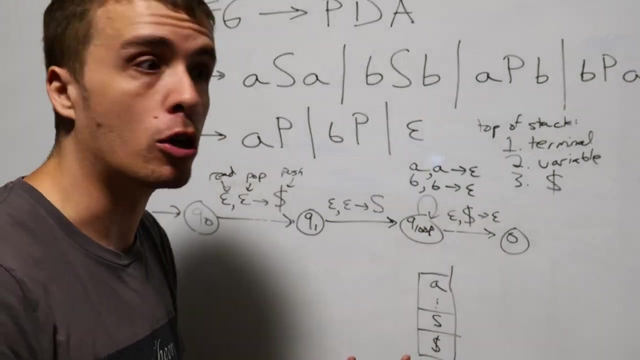 pop of each of the terminals at exactly the same time and no pushes at all. Here I'm going to be reading an A because A is a terminal in the grammar. I'm going to be popping an A and then pushing nothing. And similarly with the B because it's also a terminal. And if there were other terminals? 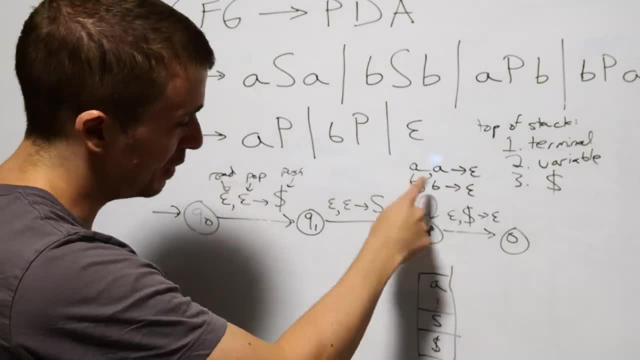 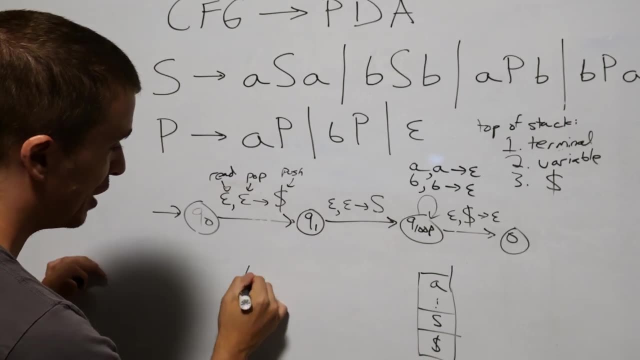 we would be stacking them up on this self-loop set of self-loops right here. And why is this a good idea? Well, think about what's going to happen. So we're going to have the input, let's say, is ABAB just as an example. If we're in Q-loop right now and we're in this situation, 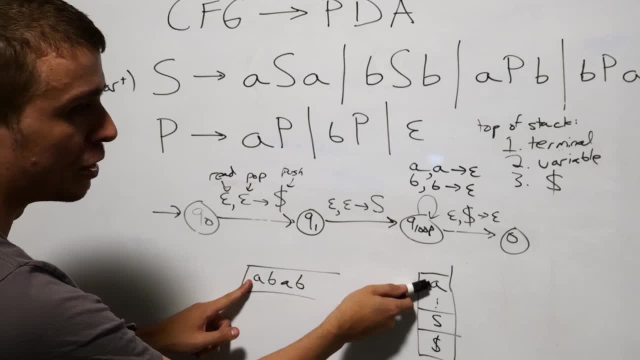 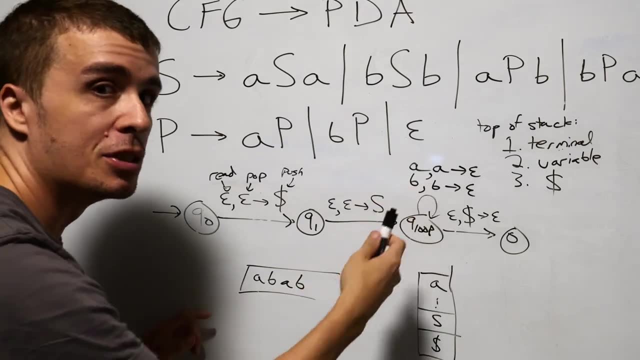 where we have an A to pop off the stack- or at the top of the stack, I should say- and an A to read. well, here I can't apply a rule and this is going to be the only transitions that read or pop. 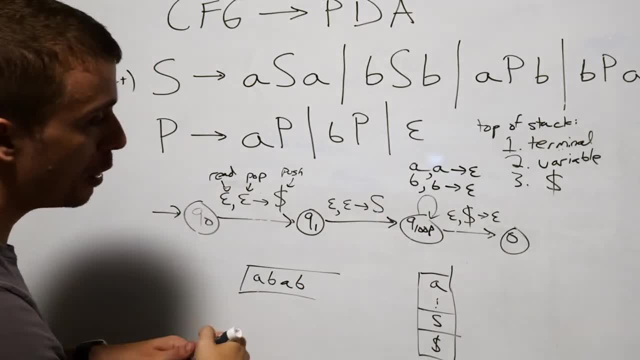 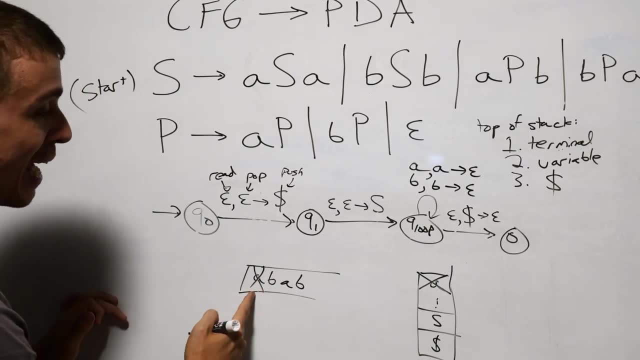 these particular terminals right here, And so therefore, this is going to be- since that's the only transition, this is going to be popped off, and I'm going to be reading this A off of the input We're trying to non-deterministically generate, because context-free grammars are. 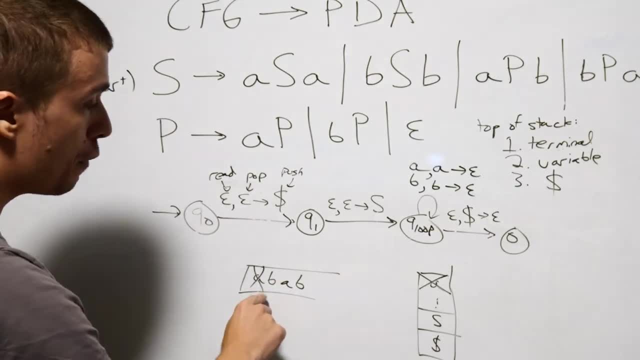 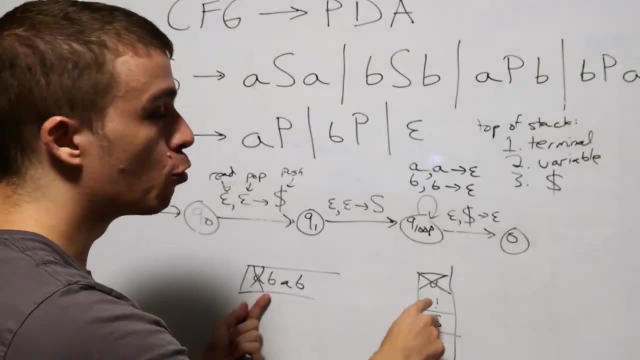 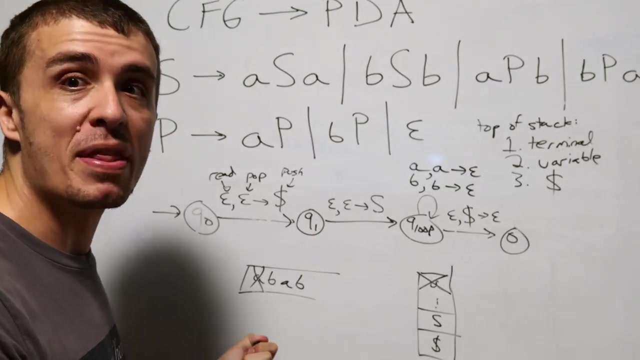 non-deterministic, and so PDAs are also non-deterministic. So therefore we're going to- and since the A in the derivation is never going to change, we're quote-unquote reading it, even though we're not actually reading it, because we're popping it off the stack. They're being dealt with. 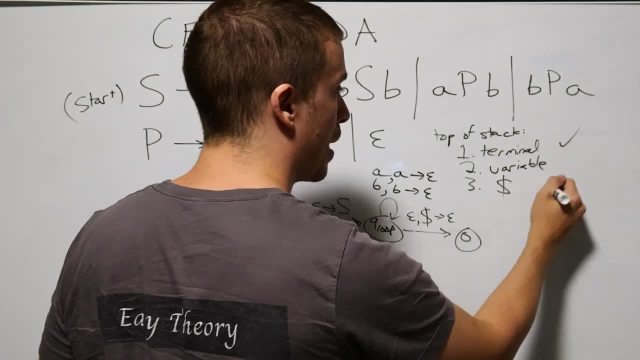 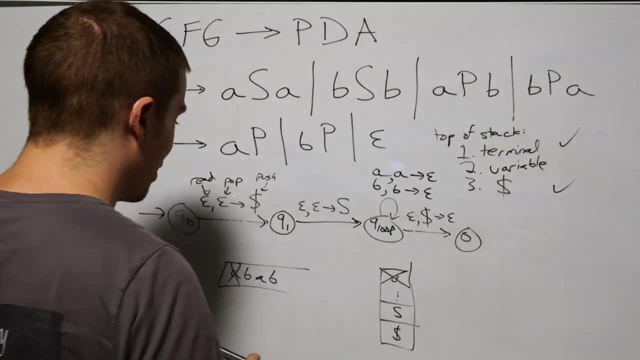 at exactly the same time. Okay, so we got the terminal working and we have the dollar sign working. How do we do the variable? Well, that's where all of these rules are going to come into play. So I'm going to try to do all of these. It's going to be a huge mess. I'm going to try to use. 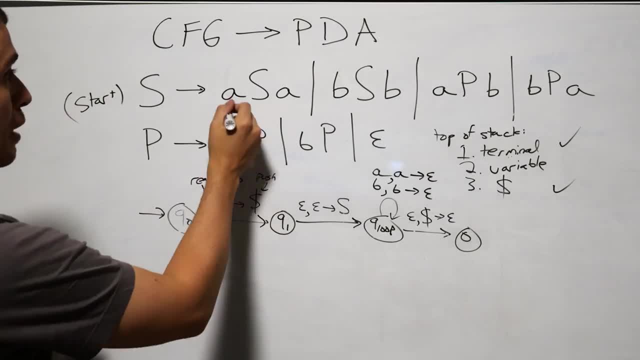 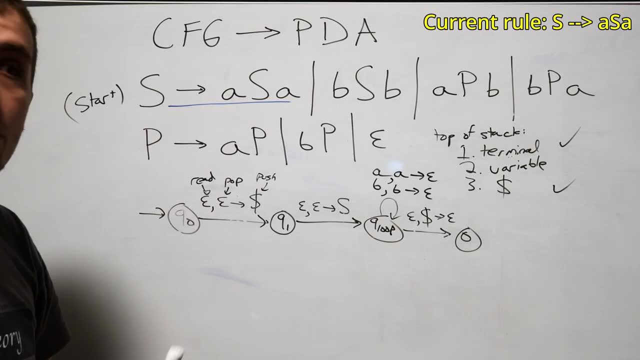 a different marker here to try to differentiate it. So I'm going to try to do all of these and let's deal with this rule first. So that's saying, if we have an S at the top of the stack, I want A S A to be replaced. So let's say that we have some derivation right here. 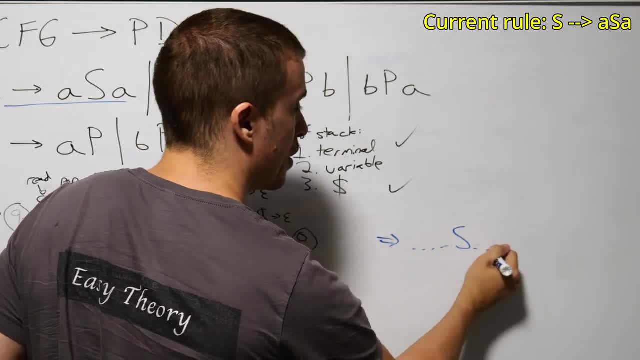 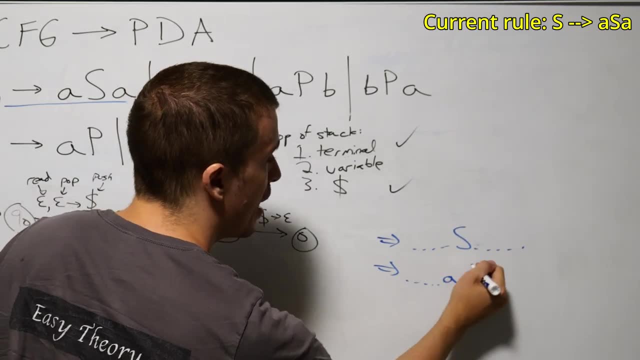 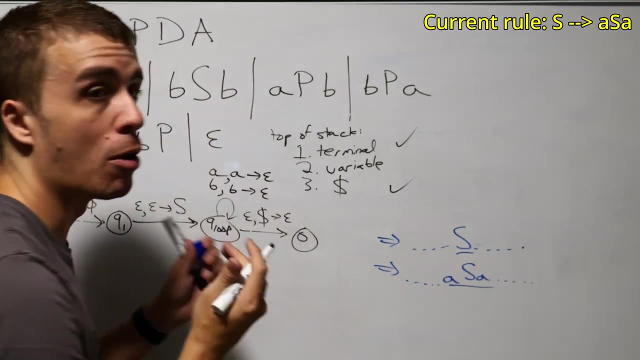 and we got some stuff and we have an S right here along with some other stuff, and then we decide, oh yeah, I want to apply this rule. So then I'm going to have some stuff- the same stuff- and then A S A along with some other stuff, because I'm replacing this S with A S A. I'm 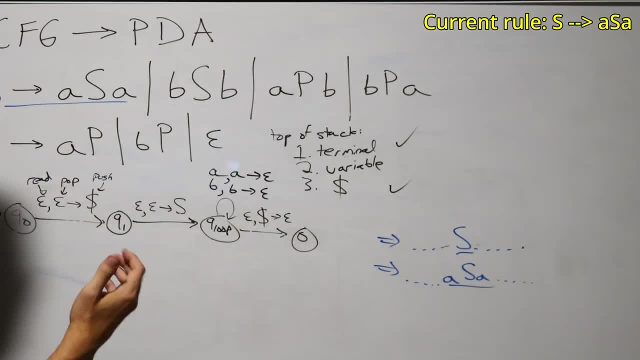 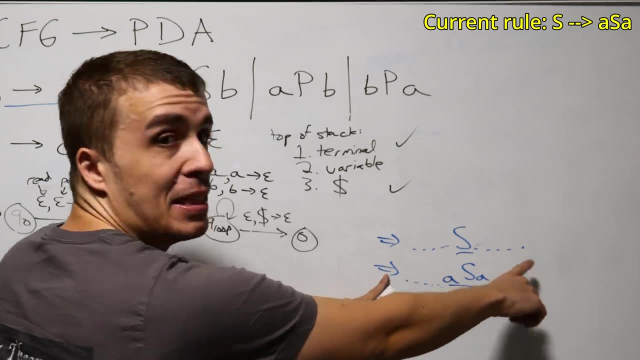 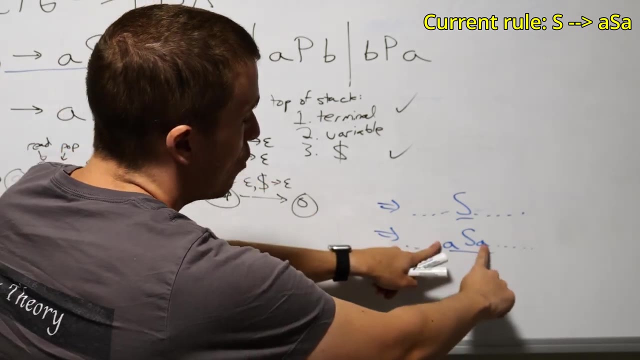 replacing it. So that means that in the grammar, in the derivation, we're replacing only this little bit right here. But if we do our little finger trick, this thing on the right-hand side needs to come down. So if we think about it this way, this A right here on the right is going to be. 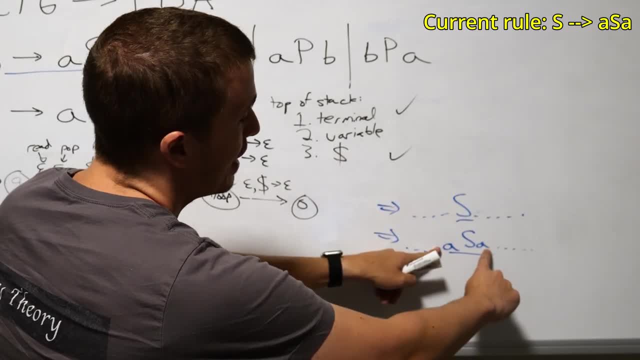 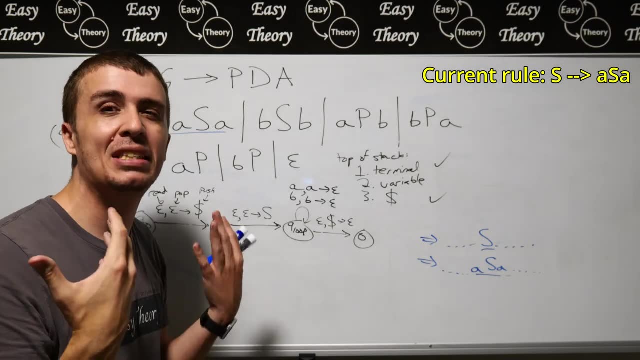 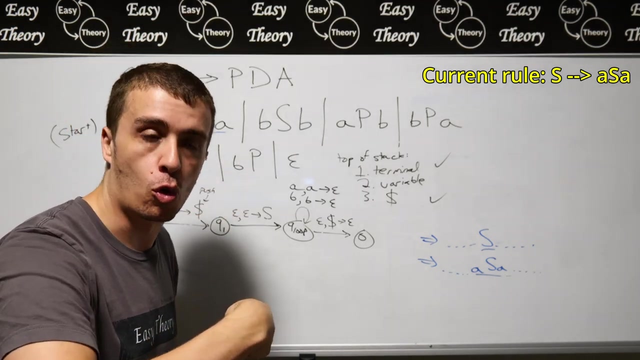 on the bottom. The left A is going to be at the very top and the right A is going to be at the very bottom. So how you actually put this particular right-hand side onto the stack is somewhat unintuitive. The idea is to take this right-hand side and push it onto the stack in reverse order. 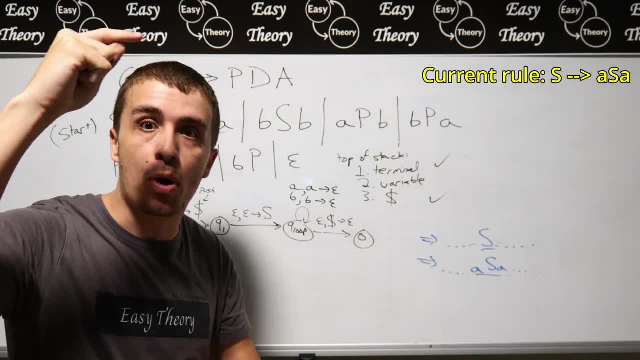 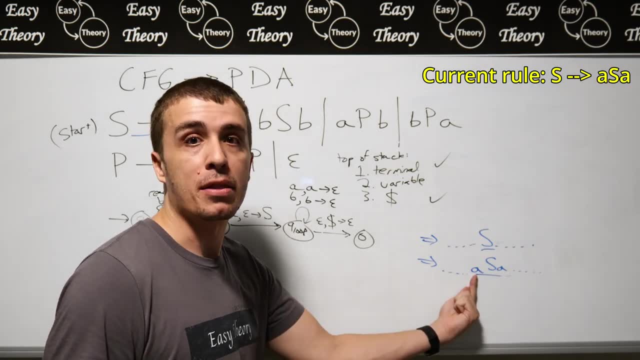 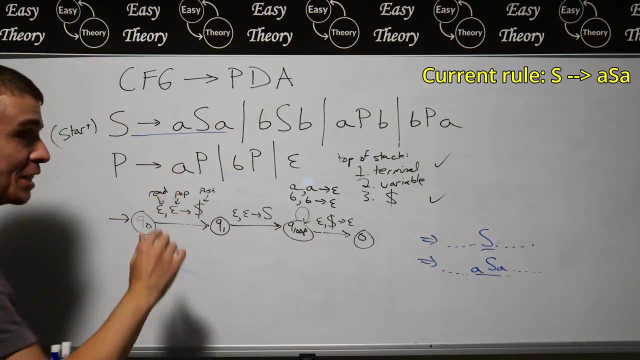 because how stacks work? the last thing that you put on is the thing at the top. So that means that this A on the left must be the last thing that we put on, not the first thing, even though the rule is completely symmetric in this case. So it doesn't really matter in this case. I'm going to 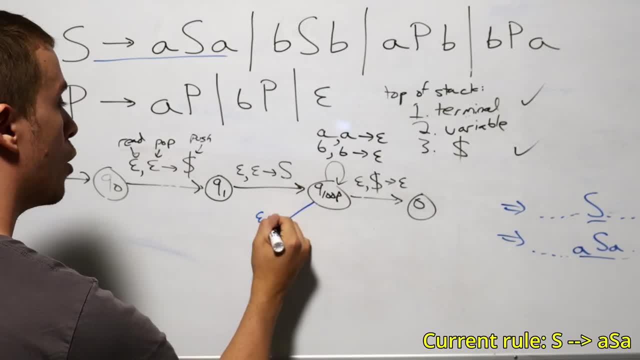 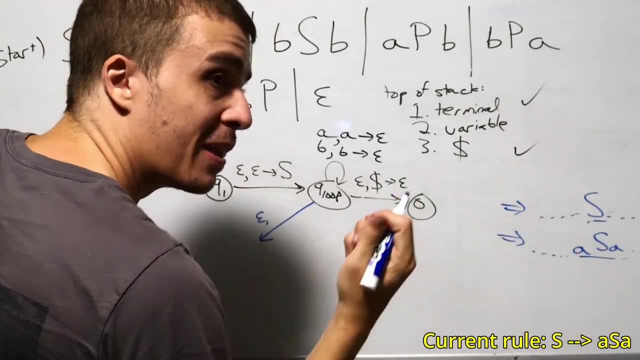 have a transition, or a set of transitions which are not going to read anything. No other transition is going to read, by the way, But we got to take this S off because we're replacing that S with other stuff, So I'm going to do it this way. There are many ways you could do this. 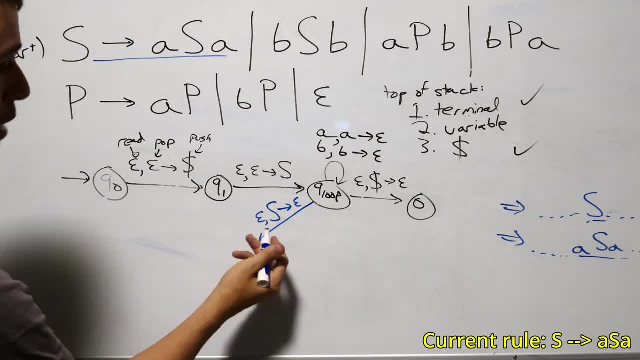 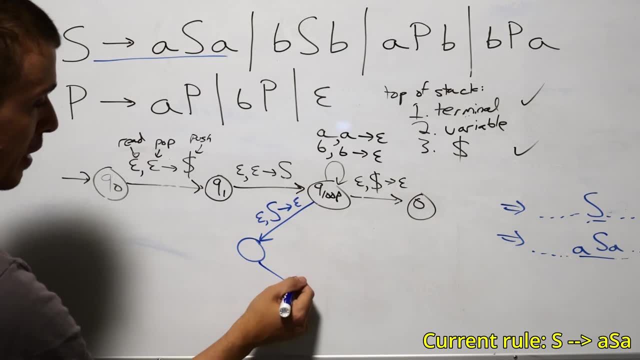 by the way. So I'm going to pop this S off, That's saying we're replacing this S with something, And then here I'm not going to name the states because there's just going to be so many- And then after that I'm going to push this rule in reverse order, So this A is going to be put on first, So that 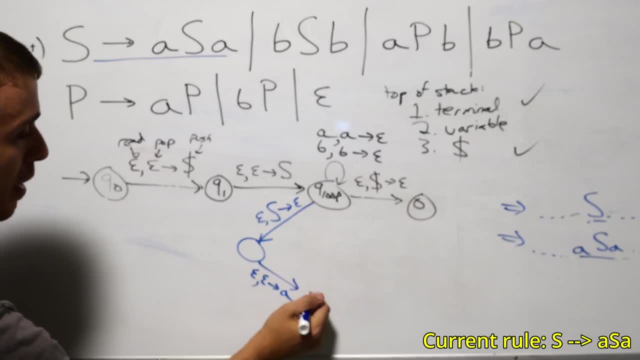 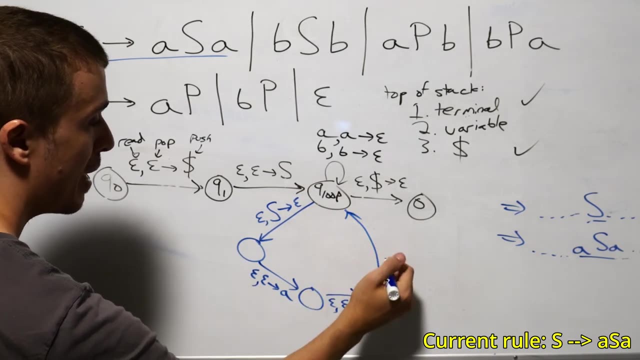 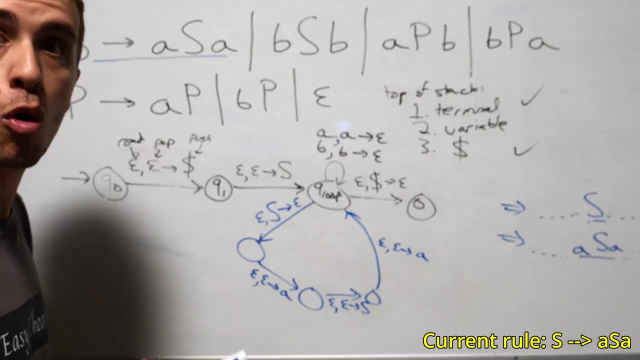 means I'm going to not pop anything. push an A and then push an S. push an S and then come back with pushing the last A. So that means that I've taken this S off and I've replaced it with the whole of the right. 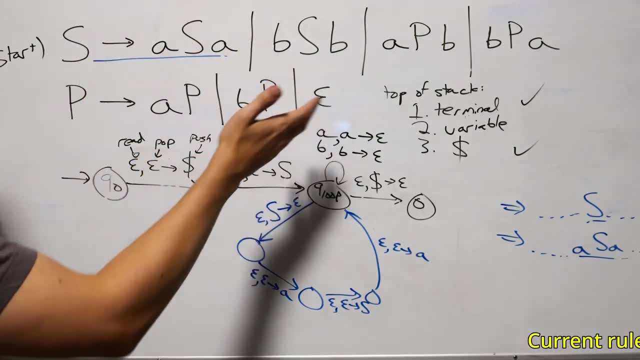 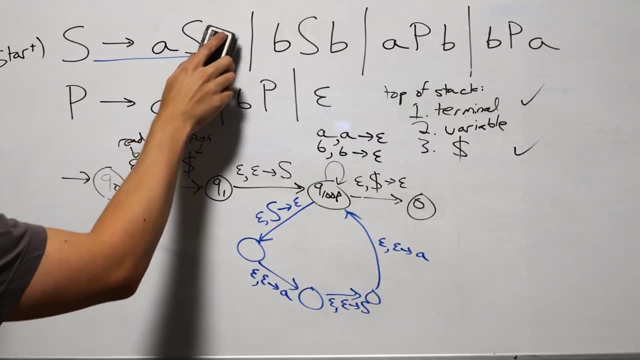 hand side of that particular rule, And then now we got to deal with all of the other rules obviously. So there's going to be a lot of things that we're going to do, So I'm going to try to make this a little bit easier. So I'm going to make this a little bit easier And then I'm going to 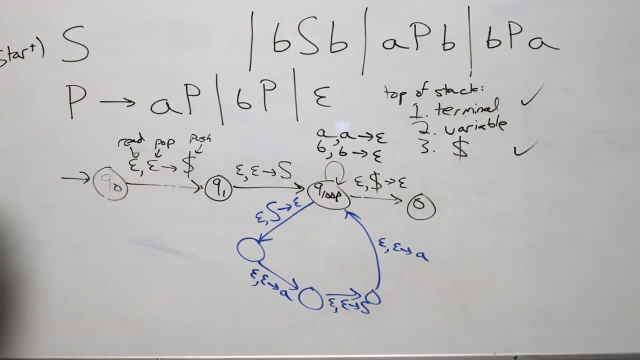 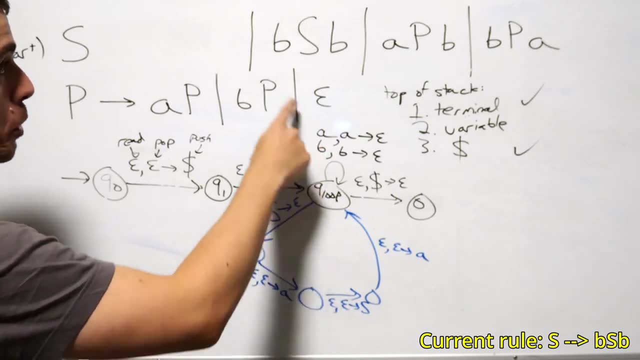 as none of a pain as possible. Now we gotta deal with this one, So S goes to BSB. The technically correct thing to do is to make a separate set of loops for each one of these particular rules, But since it's gonna be popping S off every single time, 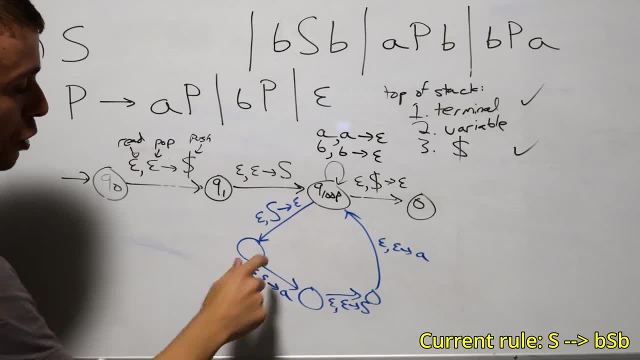 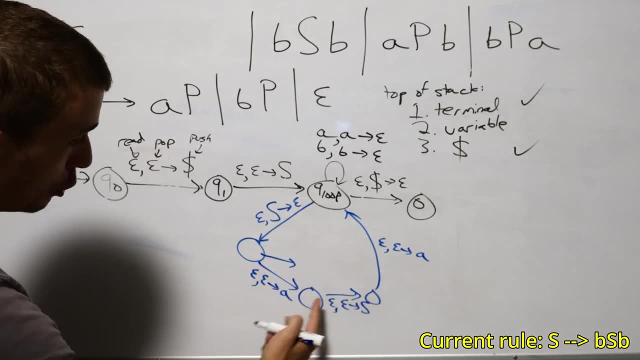 it doesn't actually matter if we just chain on this one. I can't actually deal with this for reasons that you should think about, So what I need to do is to make a different set of two states right here. So I'm going to deal the BSB rule right here. 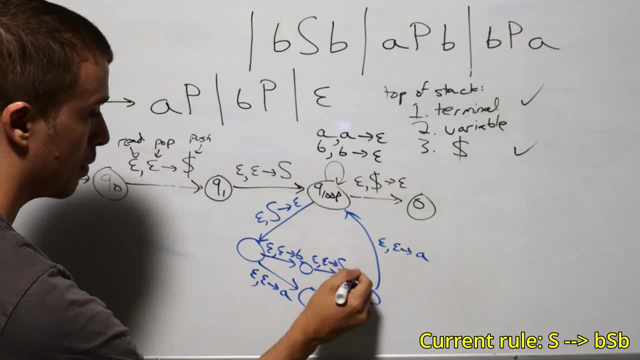 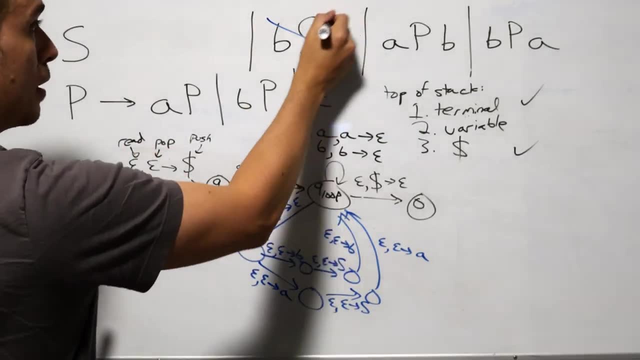 So this is going to do this, And then I'm gonna push on B So this rule is done, So I don't need to focus on it anymore. Then now we have the P rules, And so I'm going to make some more room. 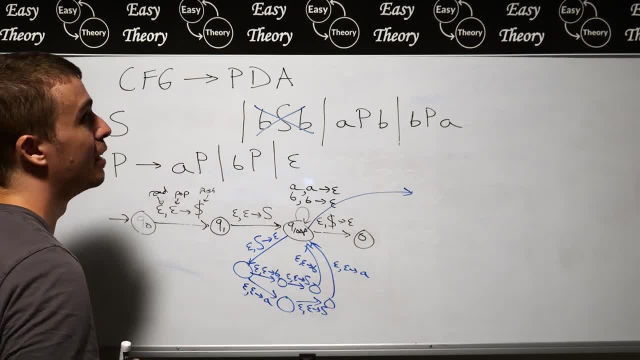 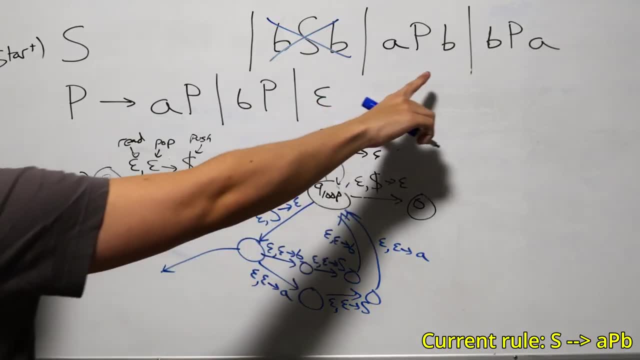 I'm gonna do a set of two more sets of transitions here, So we need to pop off S here, So that's I could piggyback off here. In fact, I'm gonna do that. I'm going to be now pushing on this one. 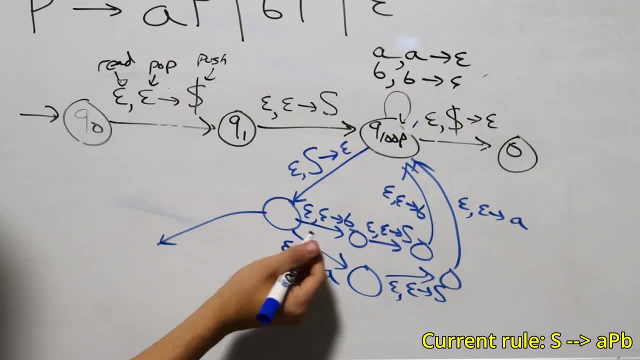 So this is the rule I'm dealing with right now, So B goes on first. In fact, I could even piggyback off that one too, but I'm not going to, So I'm going to push on the B here And then, since we're going in backwards order, 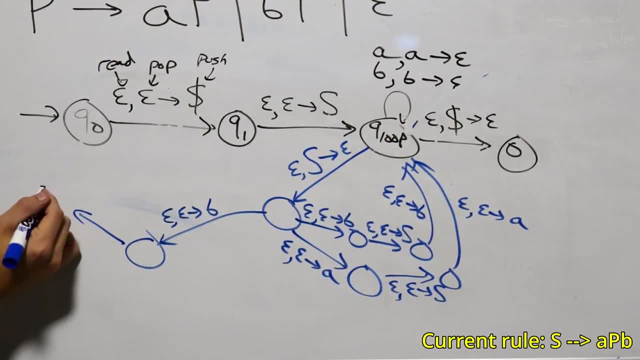 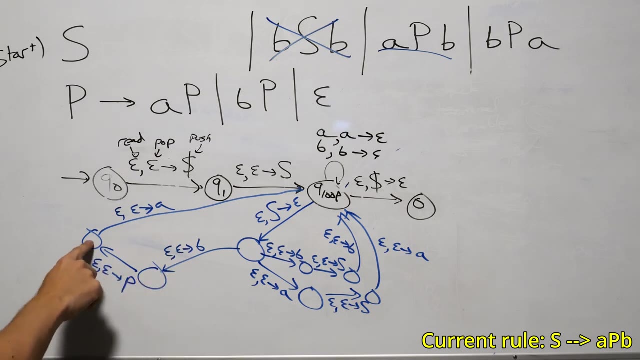 the next thing is the variable P. So P goes on. So this is gonna be a push on P, And then come all the way back on pushing A, So epsilon, epsilon, A, So that's dealing with: S goes away, B goes on, P goes on, A goes on. 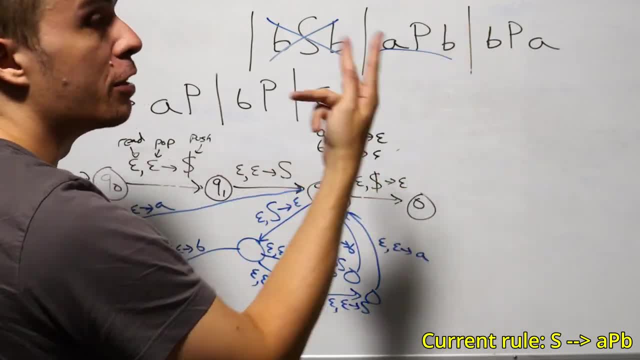 In fact, since these two rules are completely symmetric with each other, it doesn't matter which one you do first. In fact, it doesn't matter if you happen to do them in an opposite order, because they're both opposites of each other. 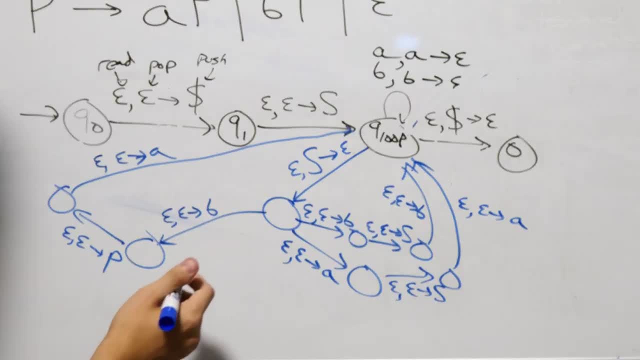 But again, we want this to be general and algorithmic, So I'm going to try to piggyback off of this one more time. So here I'm gonna do so that rule's done. I'm gonna try to do this one. 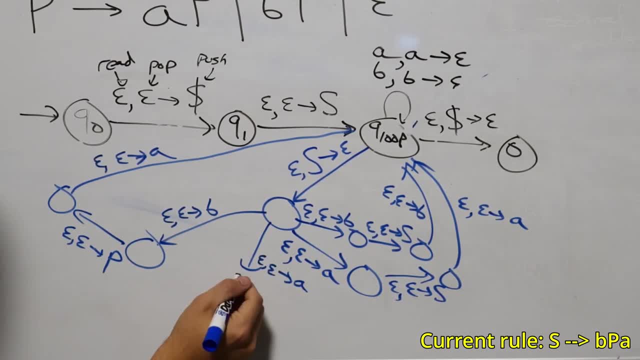 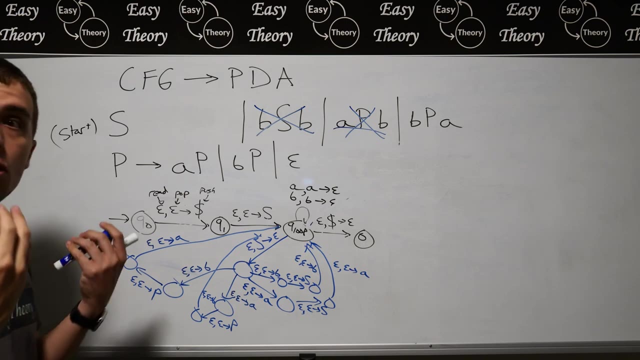 So I'm gonna do: epsilon epsilon goes to A, And then I'm gonna push on P, Epsilon, epsilon P, And then go all the way back to on pushing B. So this is getting really tight. One of the things that you should notice. 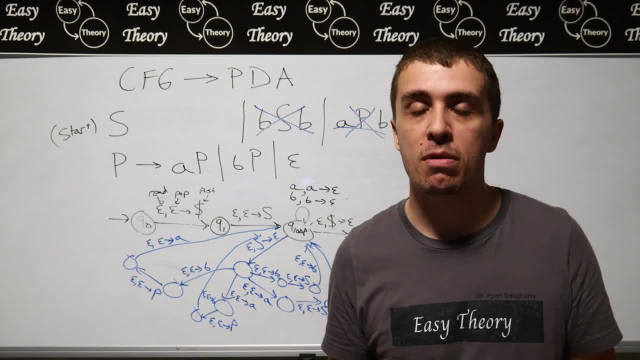 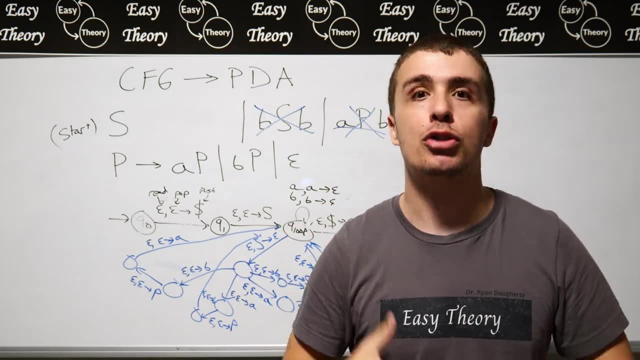 is that all of the things that we're doing here are completely algorithmic. I don't have to rely on special properties of this grammar other than what are the variables, what is the set of terminals, what is the set of rules and what's the start variable? 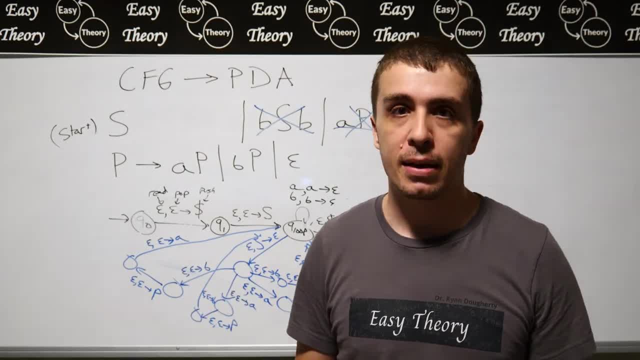 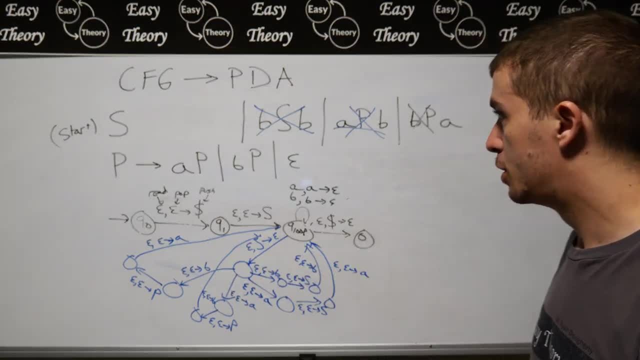 I don't care what language it is at all, I don't need all the information that I need. I don't need to know the structure otherwise. So then now we deal with all of these. So now let's deal with the P ones. 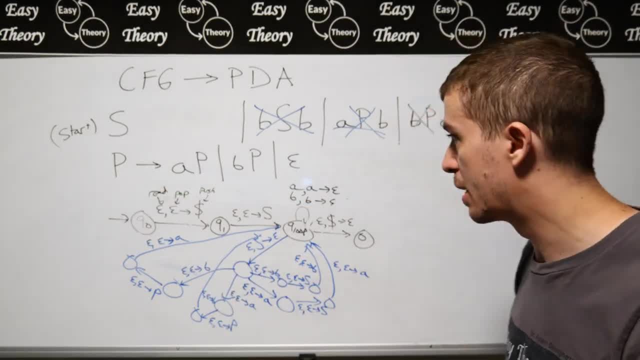 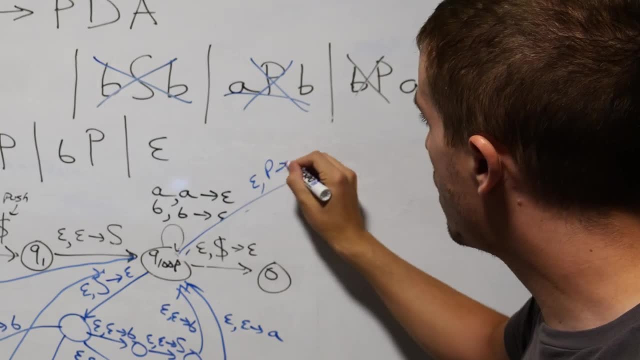 So now we have a different variable to pop off, So we can't piggyback, obviously. So that's why we made more real. So I'm going to pop off P. So pop P off, And you could try to squeeze this a little bit. 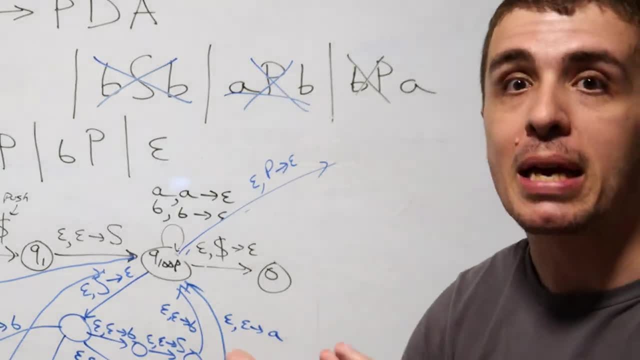 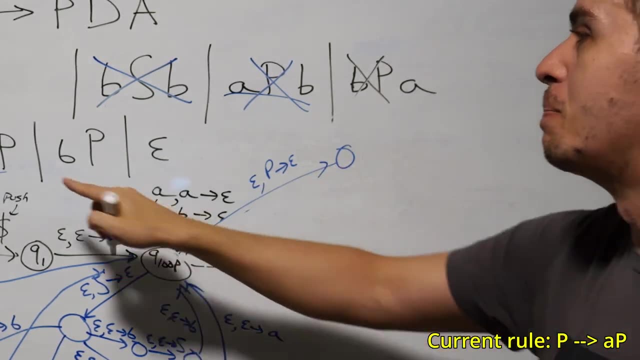 by pushing on something right here. But I'm not going to, because I want to chain multiple rules together. absolutely, put something on right here. I'm going to do this one first. So here I'm going to be pushing P back on, which is kind of weird, but I might as well do it. I'm going to push P on, so. 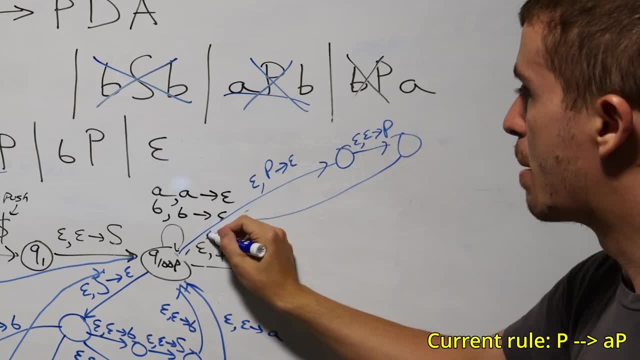 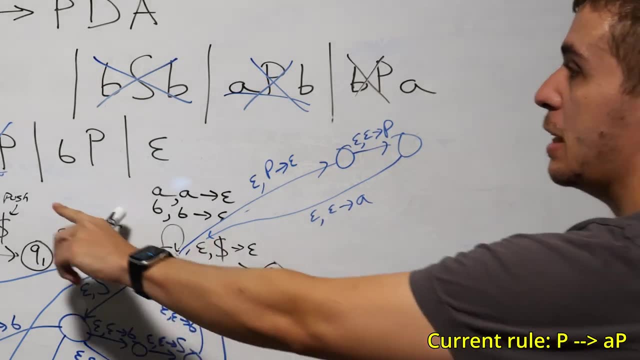 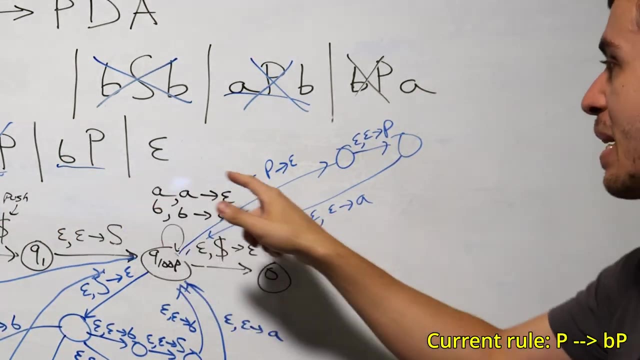 epsilon, epsilon P, and then go all the way back on pushing A: Take P off, put it back on and then push A. So I'm going, I'm doing this rule in reverse order and then now let's deal with this one. I'm going to again piggyback off of this. In fact, I can piggyback off of it completely, almost Here. 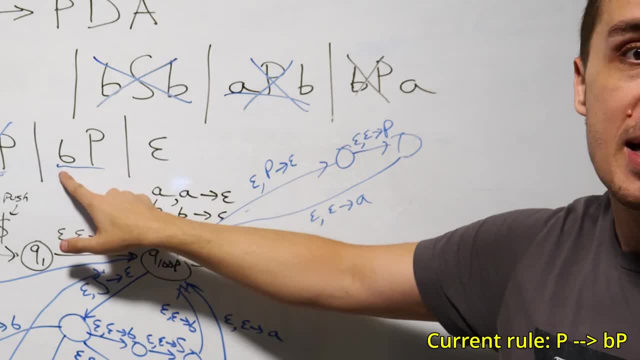 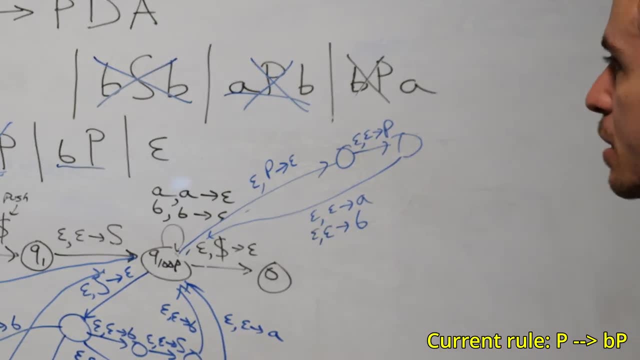 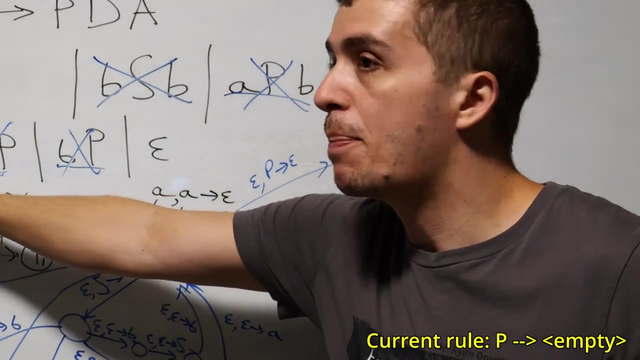 again, it's going to be popping P off, pushing it back on and then pushing now something different. So I can just add another transition right here: Goes to P, goes to B in this case. So this one's done, and then now all we need to do is to add a rule for this one, which is popping P off, and then 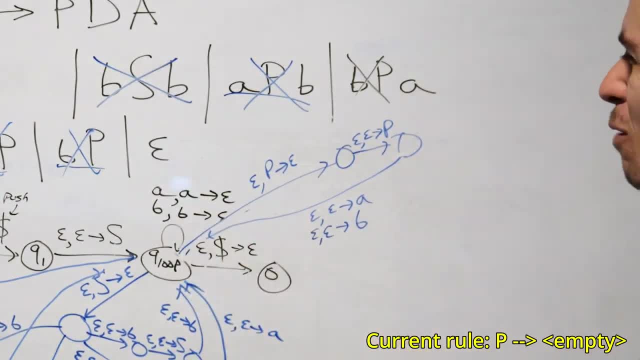 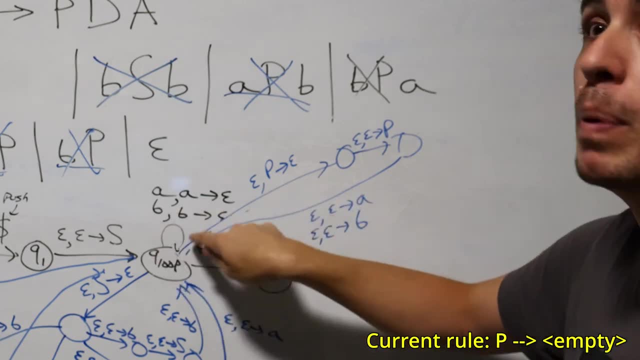 pushing nothing back on. So obviously there's nothing here and we can actually piggyback off this. Another thing we can do is to do another self-loop here, which is essentially this transition, but a self-loop, which is effectively what that rule is doing. But here I'm going to do a. 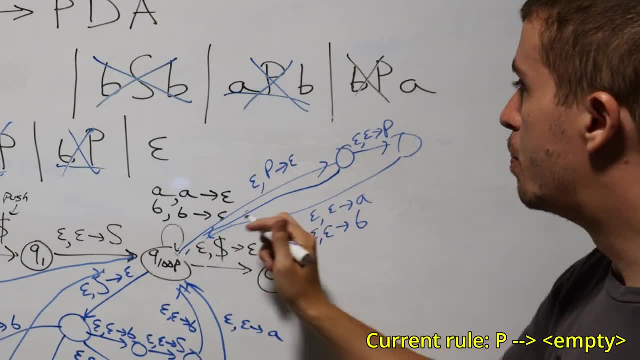 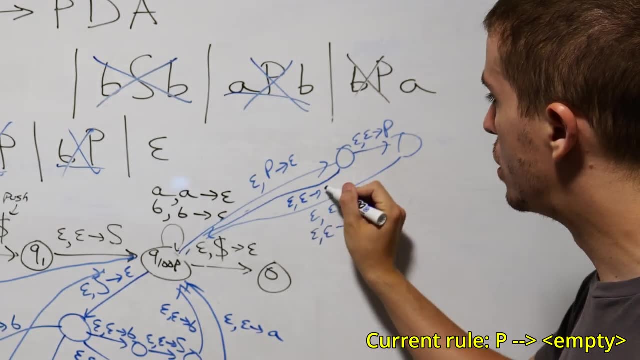 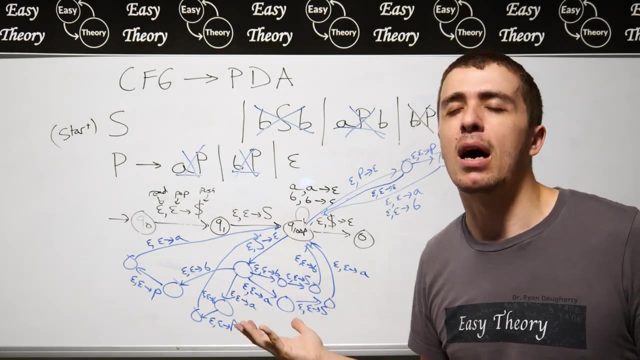 transition from here. So here it's going to be literally doing nothing to the stack, Not popping, not pushing, not reading nothing. So epsilon, epsilon goes to epsilon And laboriously, we are finally done. So we've converted this context-free grammar into this particular PDA. Obviously, there 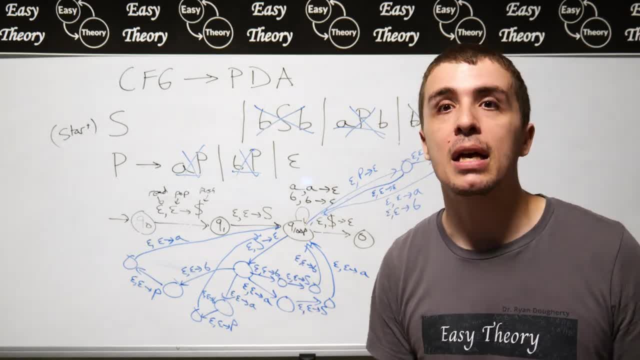 are many other ways to do this, But I'm going to do this, So I'm going to do this, So I'm going to do the, the way that this looks, it's done. So here we go. So we've cannot done in this. next, 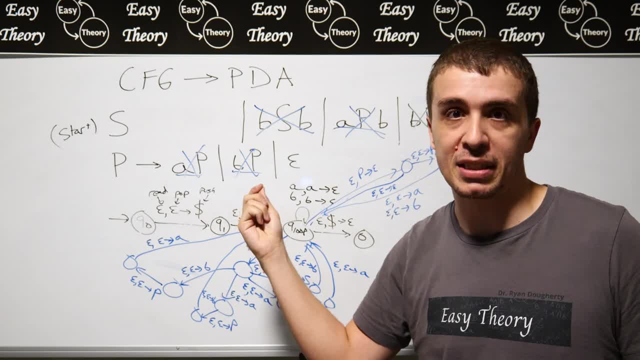 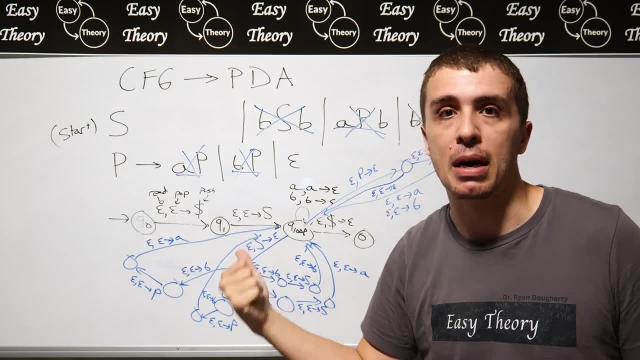 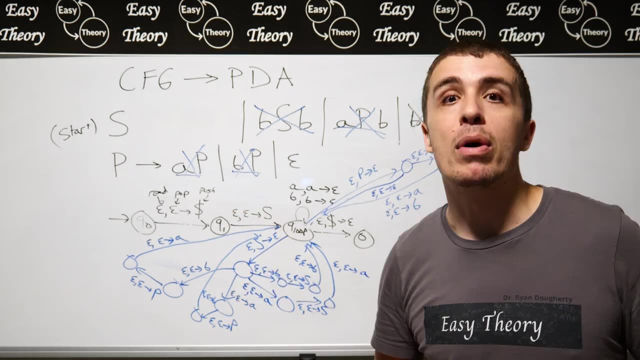 case. So I'm going to do this. we call it So here there's a box option and I'm going to do a mirror baking ability. Now, this is doing the health to the goal of choosing a particular number, and I'm going to do the same thing. So I'm going to set percentage of perception. 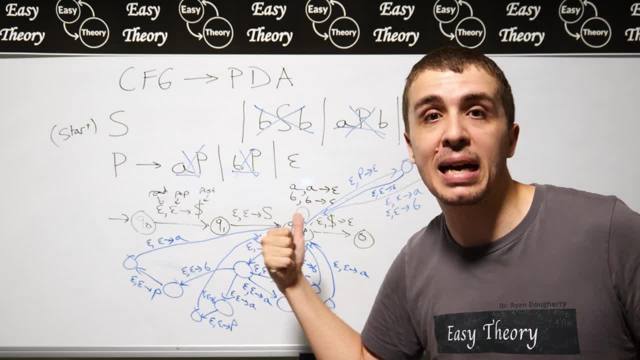 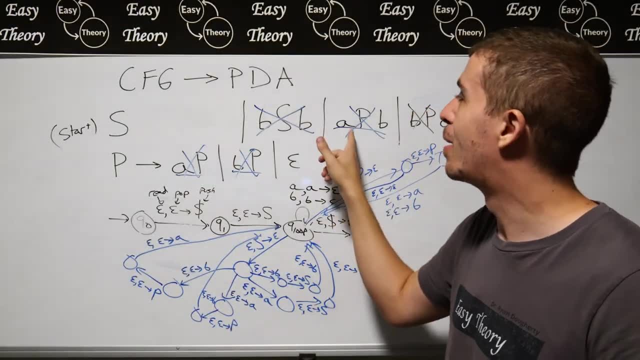 and then I'm going to set a minimum kind And now we can problema set So we can do the same again is the important point. So let's verify correctness. So if we have a derivation in the now erased, partly erased grammar, well, that means we started with S and then eventually made our way. 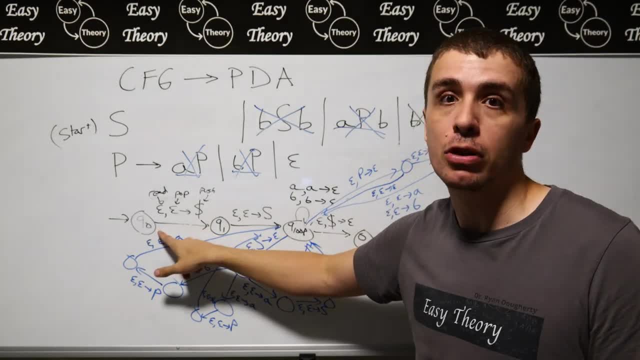 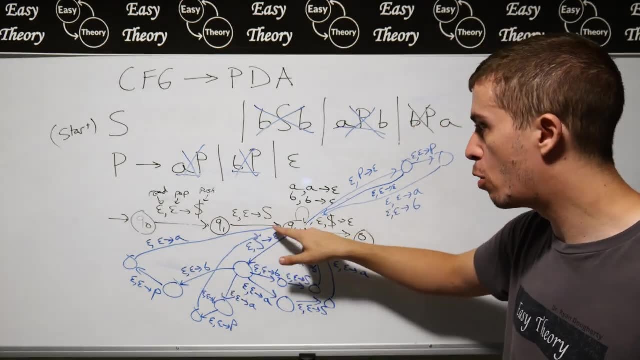 down to here via some set of rules. Does that translate to a set of transitions and accepting in the PDA? Well, let's see. Well, we start here. We can always execute that transition. Always, we can execute, because we're only just pushing stuff off. So all we need to do is to look at what rules did. 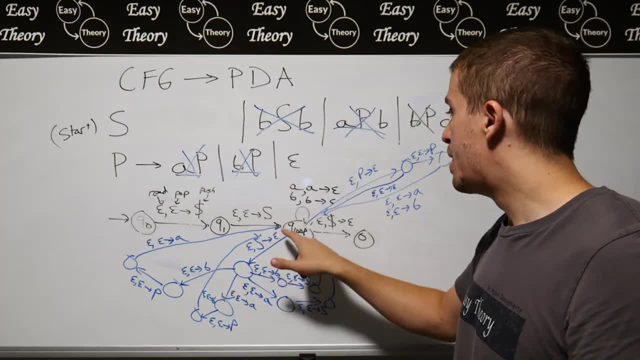 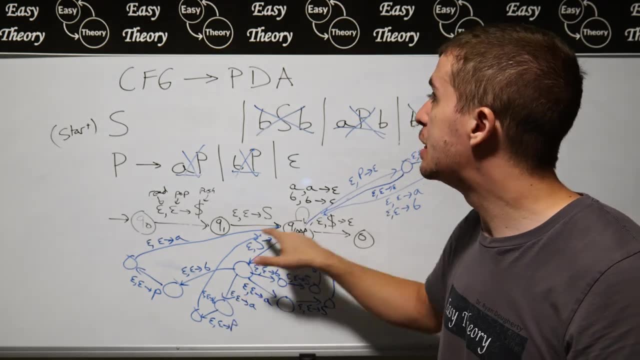 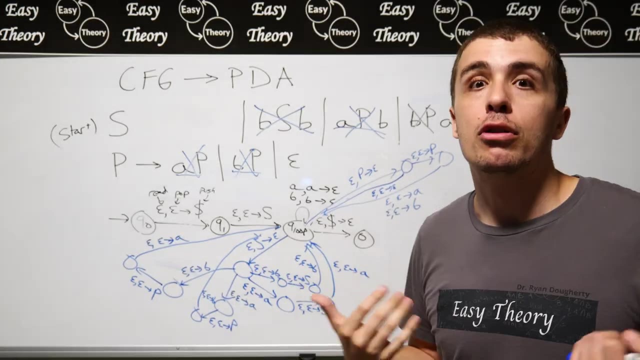 we apply. Well, if we applied, let's say, that one, that means that we, in this case, we have the choice in the PDA of applying the associated transitions for that particular rule. If we apply this one, we had a choice of applying this one. So there are many different choices that are made, but the key 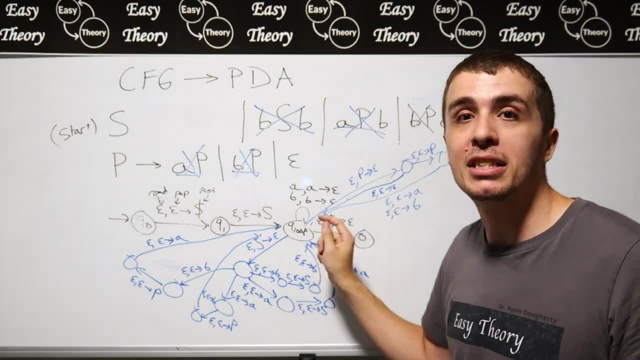 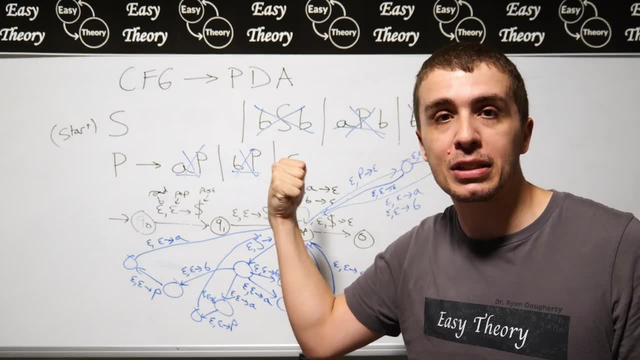 here is that these transitions are going to cause the PDA to non-deterministically choose the exact set of rules that we apply. So if we apply this one, we have a choice of applying the associated set of rules that were made in the context-free grammar and not just any set, because the PDA could 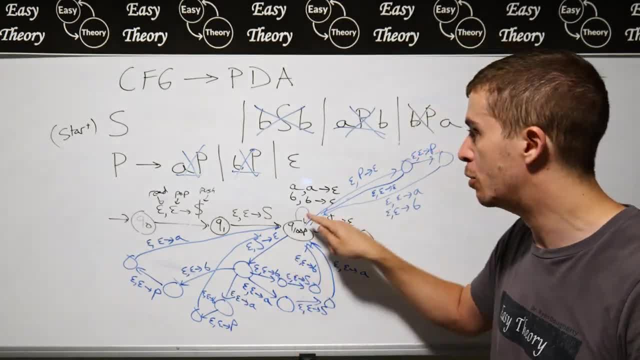 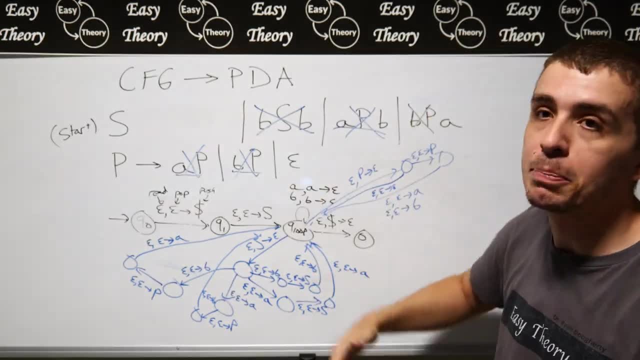 apply any of these loops any way that they want to. These set of transitions are going to stop it from just doing whatever it wants. So if we eliminated these, this PDA can do whatever it wants- and well, in fact, it can't read anything, but it could do anything it wants with the stack. 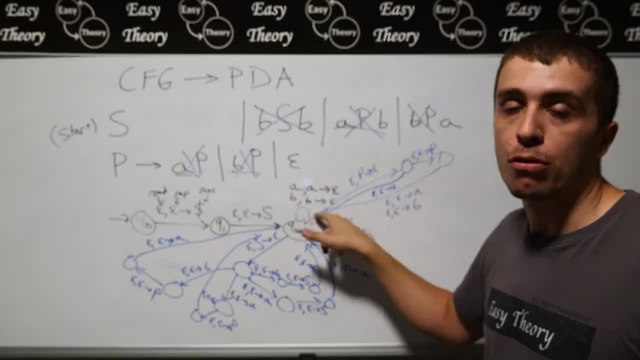 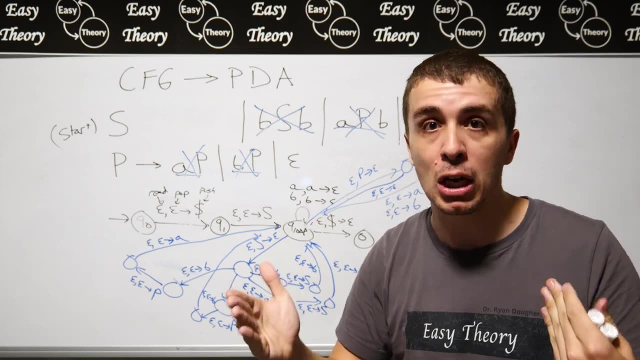 essentially That would imply that we got all the way through the characters, because if the CFG, if we had a derivation, we got all the way to a string of just terminals, which means we got to here, which means the stack had all of its terminals. 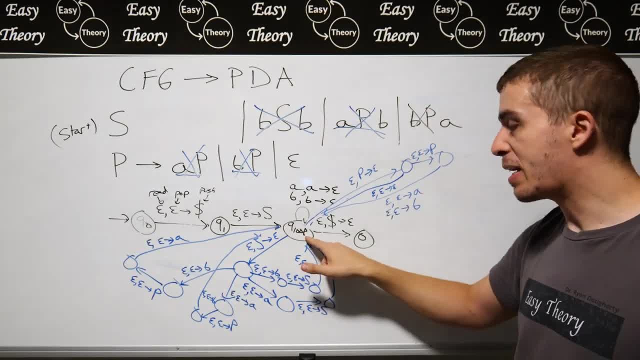 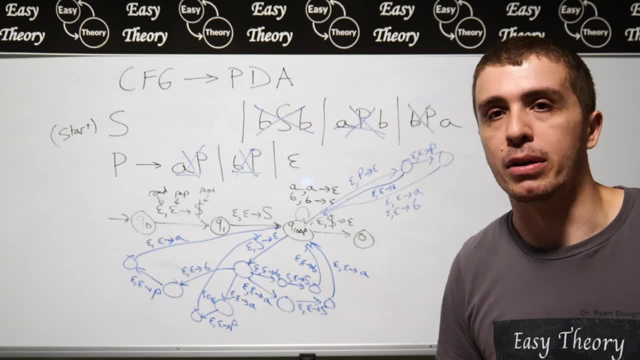 which means that we read through all of them, which means that we got to the bottom of the stack, which is where this thing comes into play, because there's no way in a PDA, at least in most models, to detect whether the stack is actually empty. So therefore, we have this bottom of stack marker to 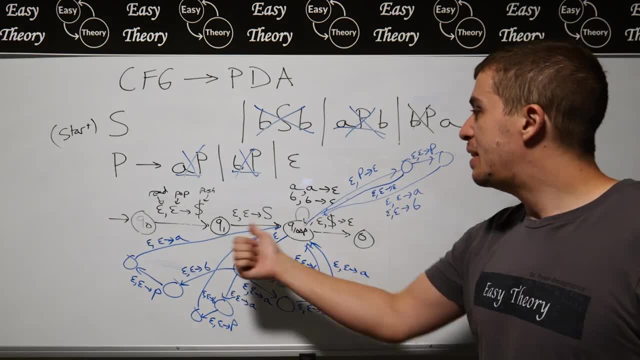 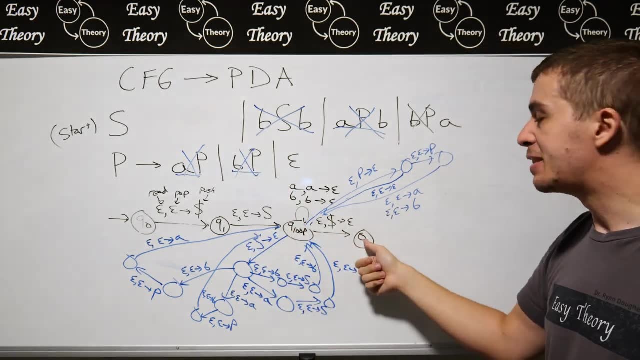 detect that for us and so now we can actually accept: Well, if we had a different string, well, if we had a longer string, then what the CFG had before. well then, that means that we get to here. we don't accept because the PDA's behavior. 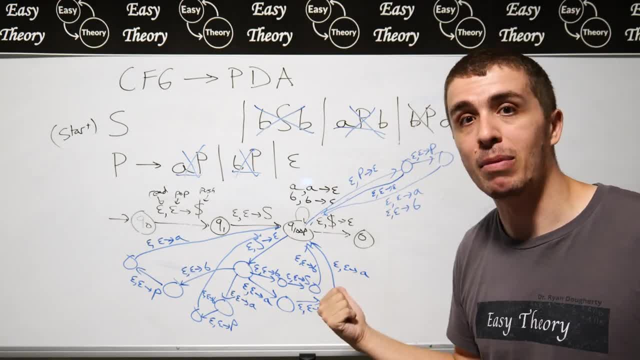 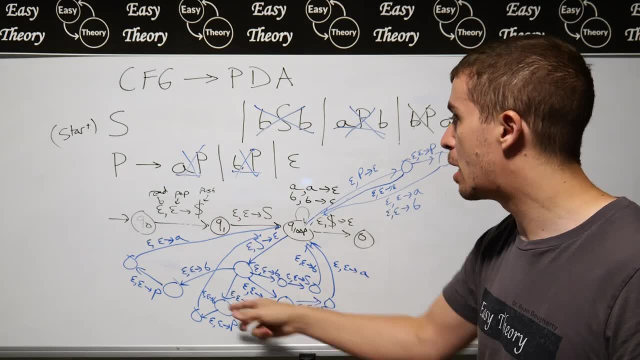 is, if you get to a final state and you haven't read the whole thing, meaning the whole string, then you don't accept, which is exactly what we want. So let's do the converse direction. If we had an accepting computation in the PDA, does that translate to a derivation in the grammar? 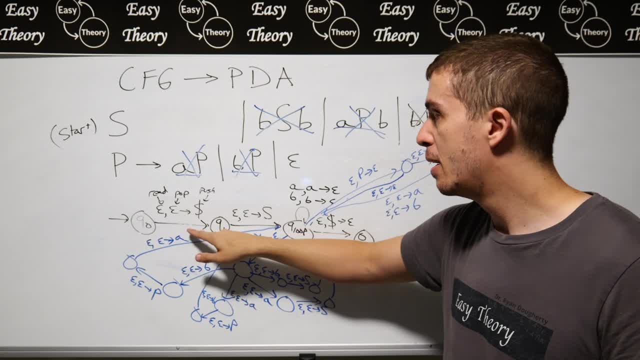 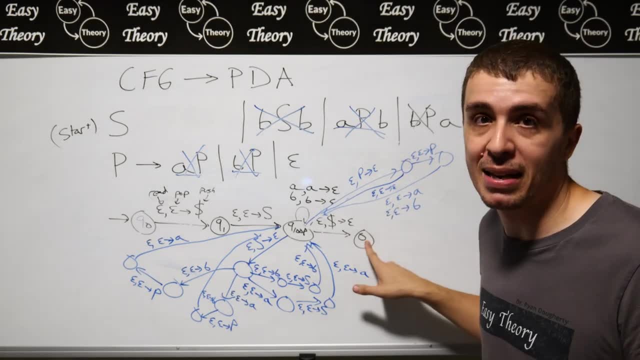 Well, the computation path must start here, because it's the start state, then it must push on the dollar sign, must push on the s here and eventually must make it here, because we assumed we had an accepting computation, which means that we must have popped off the dollar sign right here. Well, how is that going to happen? 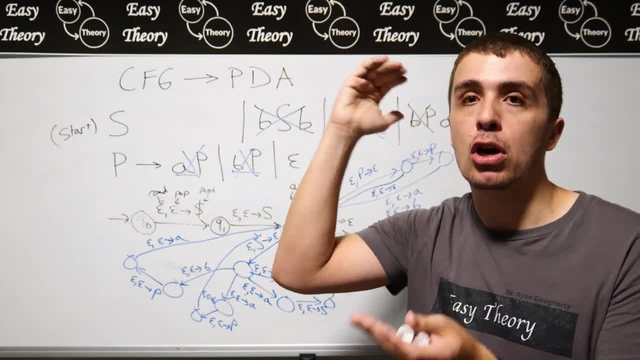 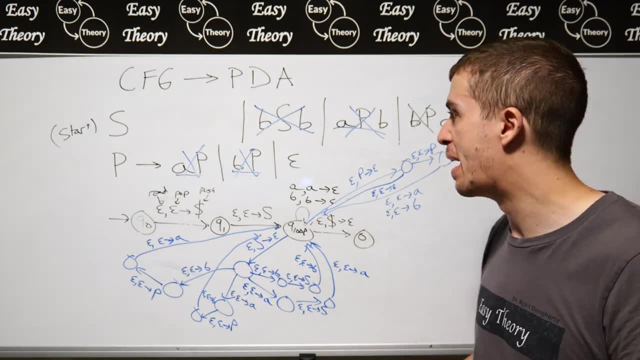 Well, that means that everything above it on the stack must have gone away, including this s. So this s must have gone away, including anything that could have happened before that. No matter what we had, the entire string was read because we got to here and we accept it. 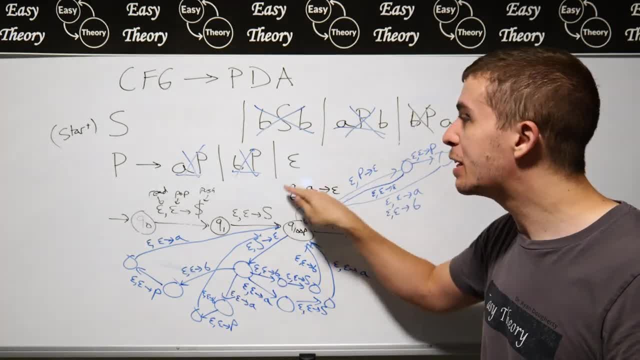 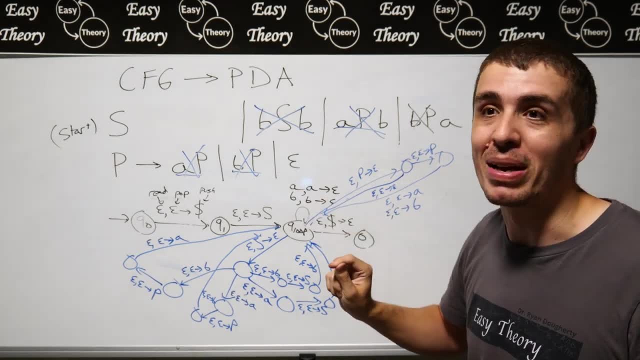 So, if we read the entire string, these are the only transitions that read, And so, therefore, we must have had all of the corresponding terminals on the stack at some point. If you look at what the paths were in the PDA, that corresponds one to one with each of the. 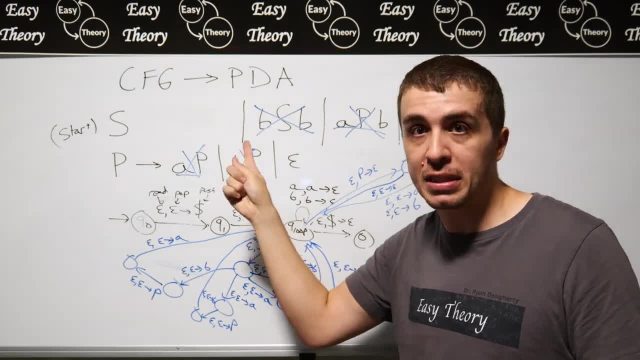 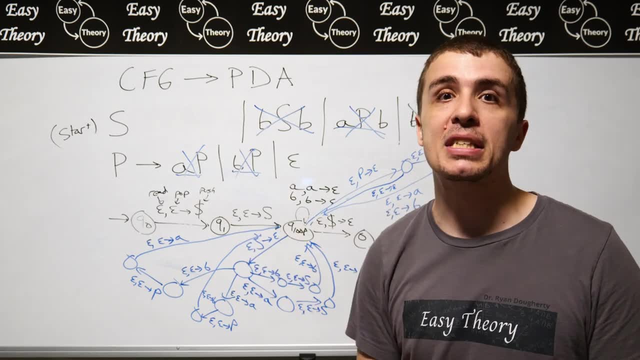 rules in the context-free grammar And so therefore, if there's a derivation up here, there's an accepting computation here, and vice versa. So hopefully that was interesting. Leave thoughts about the CFG to PDA conversion into the comments down below. As always, please like the video and subscribe to the channel. it really helps us out.